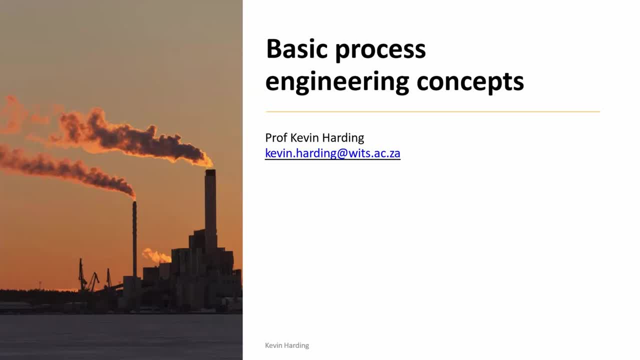 textbook. Some might be a little bit closer to the textbooks, others a little bit further away, but today is definitely linked to the textbook and, as I said, the title is from the textbook, so you've obviously seen that as well. So it is a bit of a refresher course today, so sorry for. 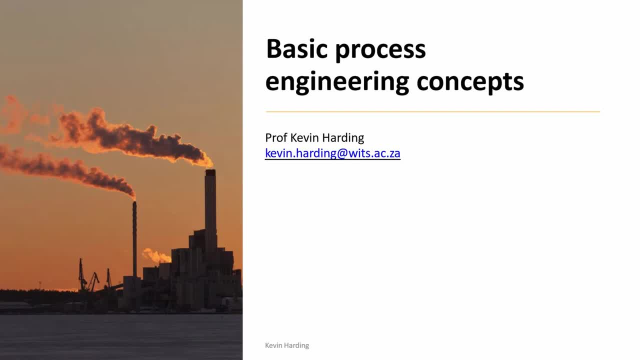 those of you that this is a little bit simple for. So some of you have probably started courses in third year, chemical engineering, where you go to this in a little bit more detail. I know the METS will also be doing some of this in their thermodynamics course, so you will all get to. 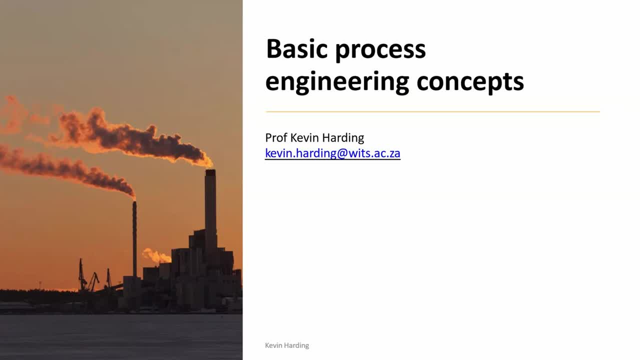 most of this stuff before. But why we want to go through this is just to clarify what exactly you need to know for this course and what you're going to pick up and what you're going to get and what you don't need to know from your other courses. So, as a reminder, the only prerequisite 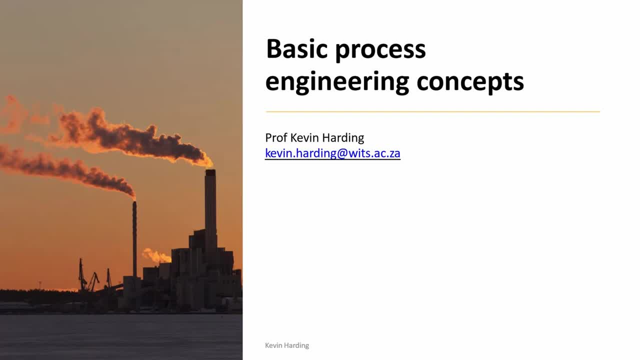 for this course was math balances, So you need to know your math, or what is that? course 2021, CHMT 2021-2025, the two courses that you did. that was the only prerequisite, But there are some concepts that are going to be involved in environmental engineering that go a little bit. 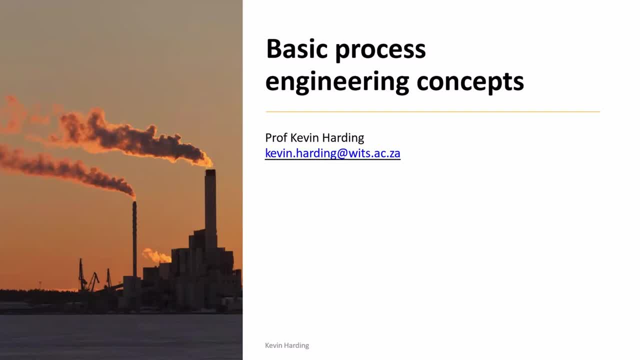 beyond that. So that's what we're going to cover today, and just to highlight what exactly it is that is going to be examinable. So just that's the key part. what is going to be examinable in this course? The first. oh sorry, I'm not clicking through my screen. 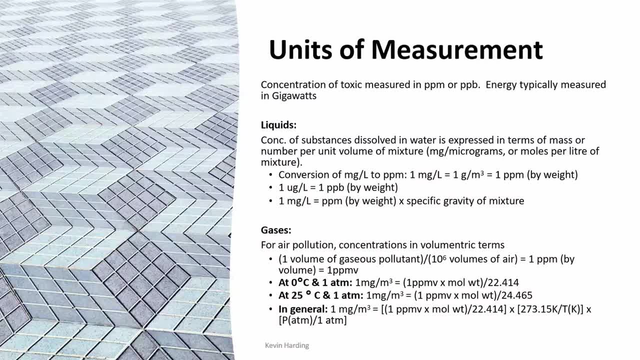 So the first issue that is going to be important for us in environmental engineering is the units of measurement. So we've all seen, as I've already mentioned, that a lot of things are going to be in gallons per litre, gallons per pound, pounds per cubic foot and all those funny units that the 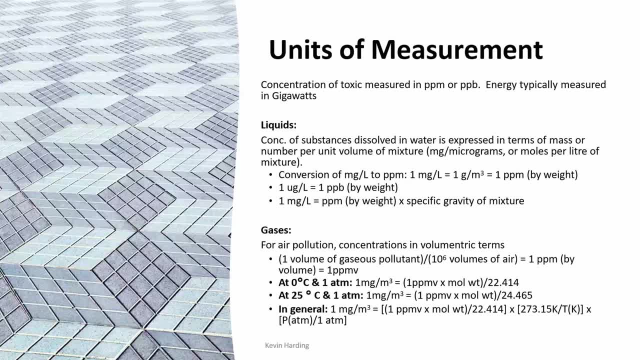 Americans seem to like the imperial units And unfortunately, they are going to sneak their way in, So we do need to remember and remind ourselves exactly how to do units of measurement. So the first thing that I want to highlight today is: please, can you go back? I don't know, I can't recall where you did unit. 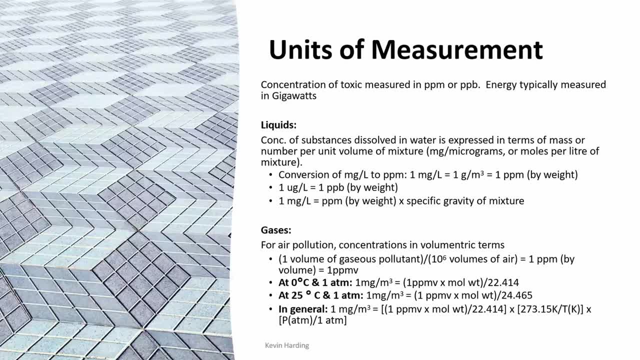 conversion. So please go back and have a look at how to do units, unit conversion. OK, in particular in the environmental engineering world, we are going to be working with two things: the liquids and the gases. And, in particular, of particular importance- sorry- is how we measure concentration. 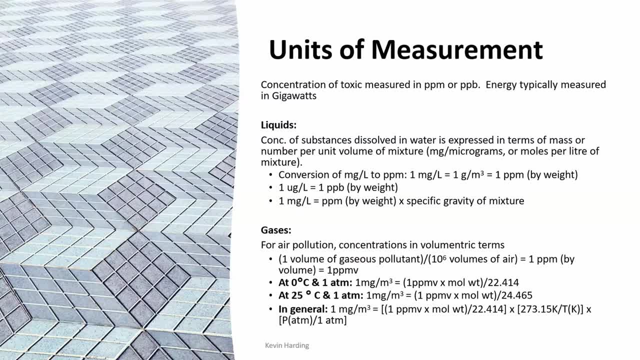 So the first one that we are going to worry about is parts per million. So just to check here, we've got this on the top here: parts per million. Sorry, I just want to get something here quickly. So, as I say, first one is parts per million. 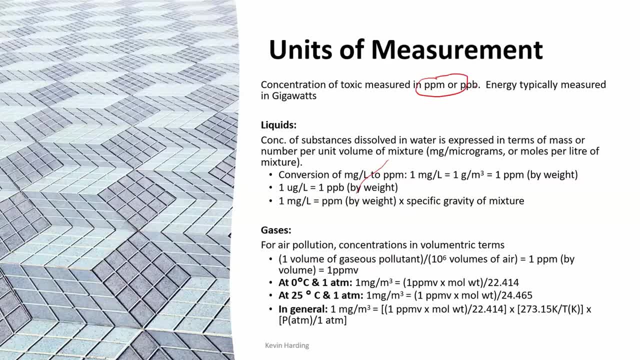 So we need to worry about what is a part per million and the second one is parts per billion. So please just make sure that you understand what those mean. So what is that? How do we get to that? So the easy way to think of that is that when we're looking for a liquid, 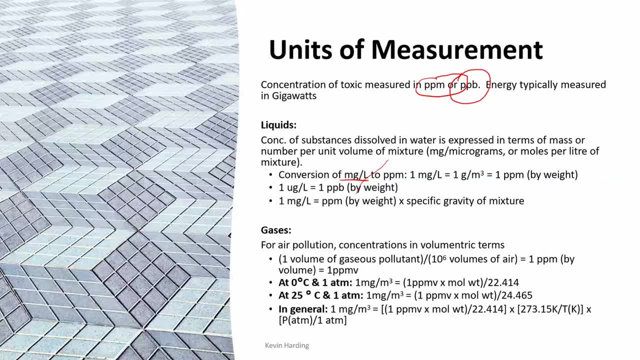 the conversion is a milligrams per litre is the one that is easy to measure in the lab. If we want to convert that to a parts per million, one milligram per litre is one gram per cubic metre, which is equal to one part per million. 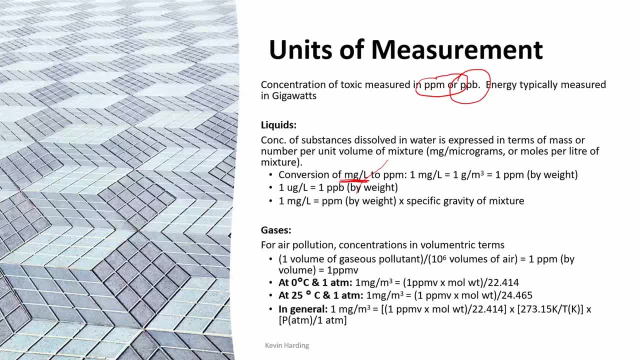 So that is by weight. I've forgotten to change this, so let me just find where my pen is. This should be the symbol, for it's not necessarily a U, that is a microgram. So one microgram Microgram per litre is then one part per billion by weight. 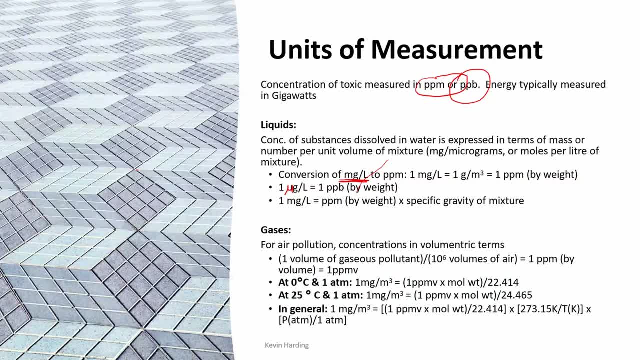 Okay. so if we want it by weight, in terms of sorry- I'm echoing sorry- We can also change that by sorry. that should be by volume, So I need to cross that out. That's not by weight, that's by volume. 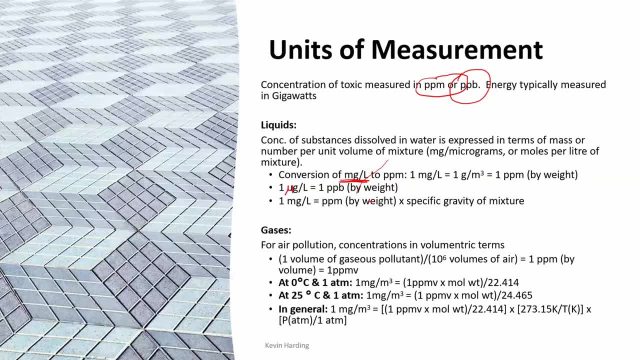 One milligram per litre is equal to a part per million, which we said in the first line. If we multiply that by specific- sorry, that is by weight- One milligram per litre is equal to one part per million by weight, multiplied by the specific gravity. 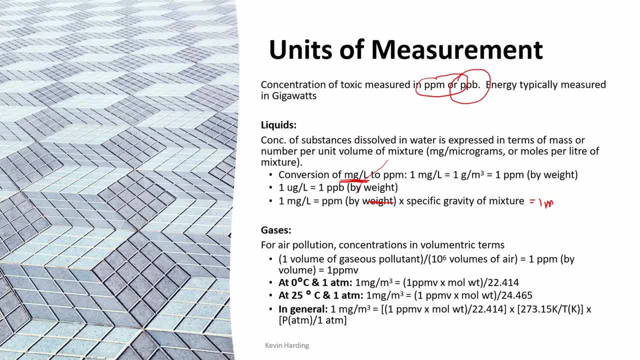 will equal to one part per million by volume. Okay, so that is for the liquids and that's the important one that you need to, that you do need to know for this course. So please make sure that you can convert those units for liquids. 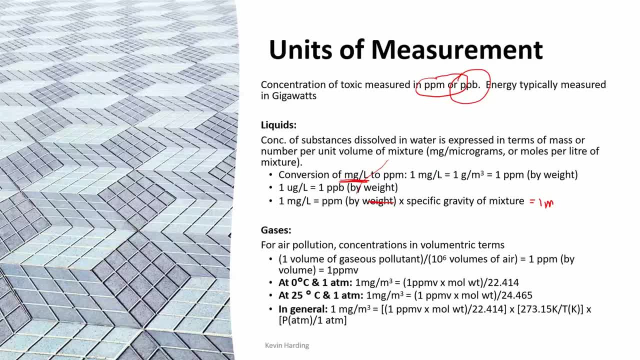 In the same way we need to know what the concentrations are for gases. So this again is fairly- I hope it's just a summary- for for all of you, particularly for air pollution, We want to know what the concentrations are. So the volume of gaseous pollutants divided by 10 to the sixth volumes of air will give you one part per million by volume. 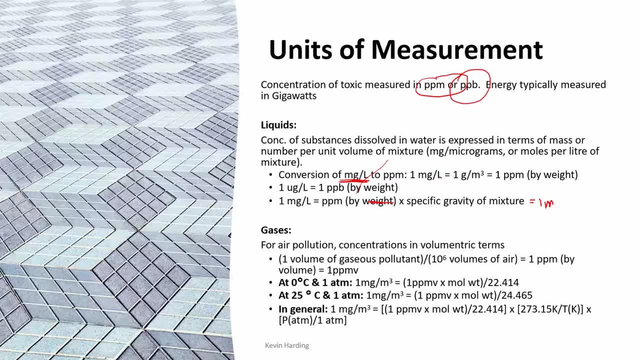 Okay, Liquids. it's very rare to have it as a volume. It's almost always per weight. So I think I'm going to actually, in the updated notes, I'm going to probably delete this, but just remember you can get it. you could convert it to a volume, but it's almost never given. 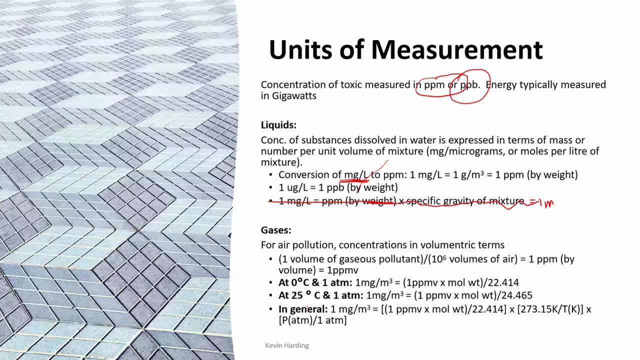 It's only for gases that we have the volume, As you all remember from your PVNRT laws in chemistry, if we change the temperature or the pressure. so if we're looking at zero degrees or 25 degrees Celsius, we are going to have to change that based on compressibility of gases. 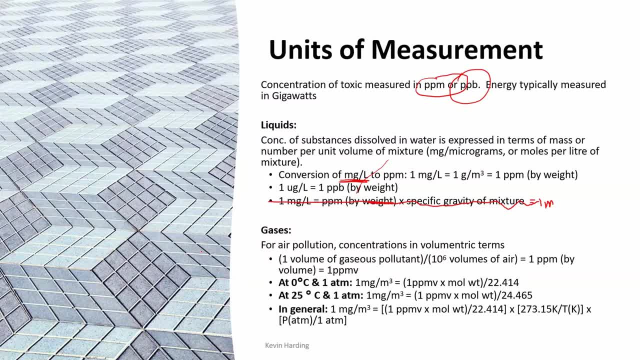 So gases being compressible, we will have a different ppm by volume. Okay, And you have tight questions that we'll be looking at that. In general we've got the one milligram per cubic meter. We can times that by the molar weight at 22.414. 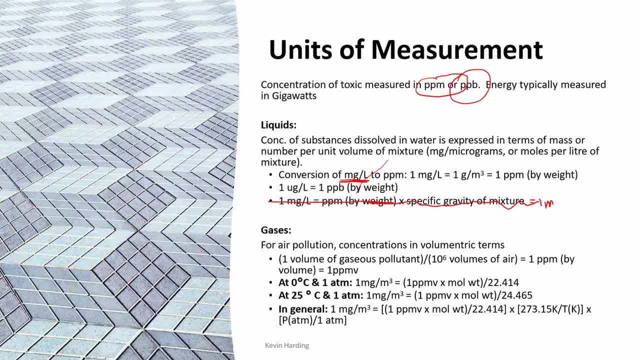 I hope that you all remember that. Okay, Remember that number from chemistry for a volume of gas multiplied by the temperature and the pressure, So you can get the ppm's in general for gases. Okay, So the takeaway message from this slide is that you need to know how to get parts per million or billion for liquids. 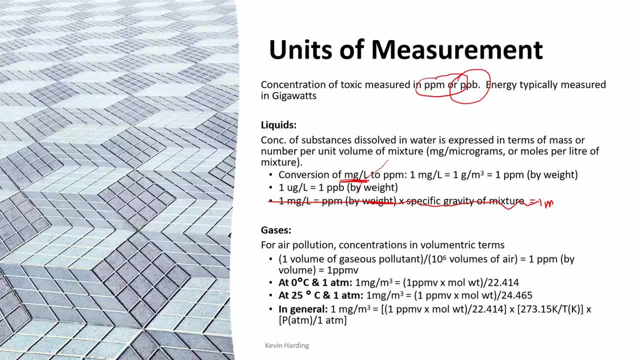 which will be by weight, and for gases which will be by volume, The gases. you need to be able to look at that at different temperatures as well, based on the PVNRT type logic behind it. Okay, Are there any questions on that? 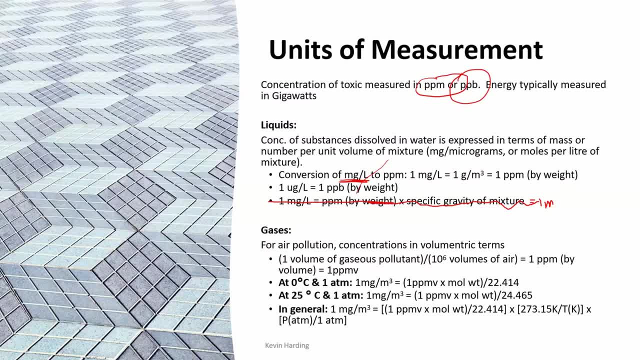 On what you need to know. I will also be requiring you to know the general unit conversions. So how many inches in a foot? how many gallons per or not? how sorry, I don't need you to know them. I need you to know how to convert them. 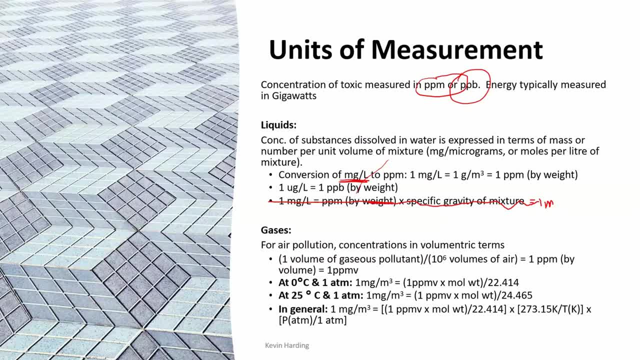 So feet to cubic to meters, inches to feet, feet to inches, obviously, gallons to liters, cubic meters, those sorts of things. Okay, For a touch, you will be looking them up. You've got your own notes where you can look them up. 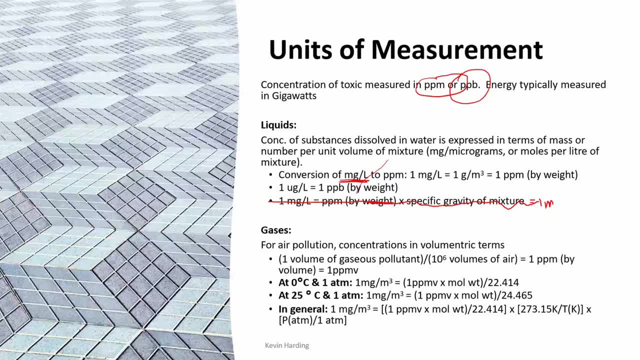 Okay, For a test or an exam, I will give you the unit conversions. Okay. So, reminder, I will give you the unit conversions for these type of things in a test or an exam. A touch, please. you need to look them up. 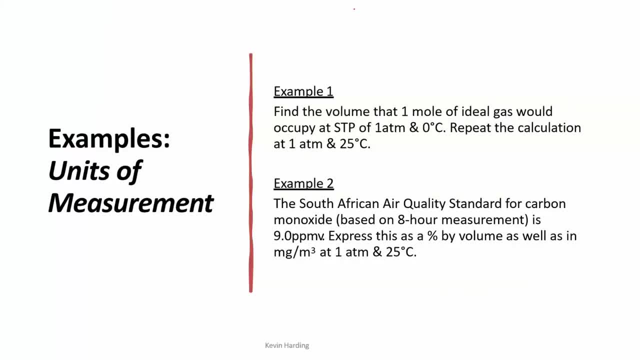 Oh, sorry, now my slides won't move over. Okay, So how can I ask you these questions? So from this- so it doesn't mean I'm not going to ask you general knowledge questions in the tests or assignments, tests or exams, rather, 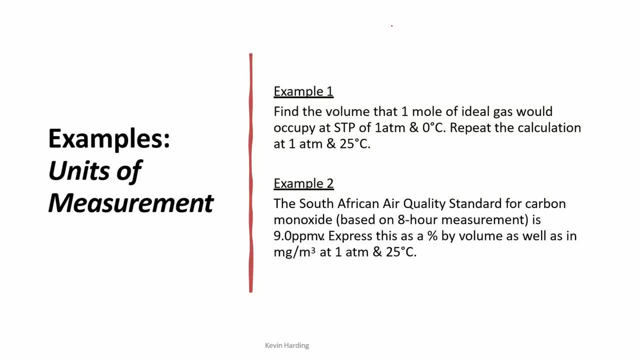 But from this course- sorry, from this week onwards- you're going to start seeing more questions, like you're probably used to in engineering. So, find the volume, find the mass, what is the size, the length, the cost, those sorts of questions. 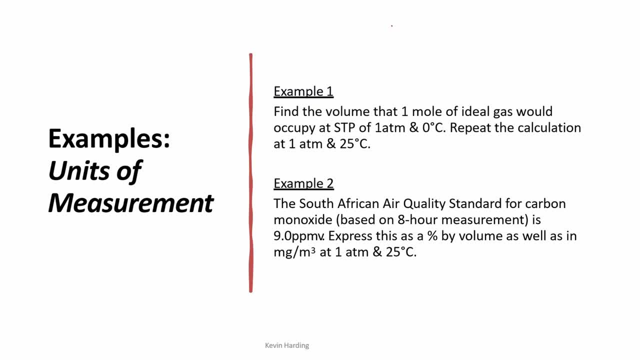 So today I'm not going to go through these examples. I'm going to leave you to have a look at these examples in your own time. I will probably not be giving you the solutions to these examples in the notes. So, the notes, I will not be giving you the solutions. 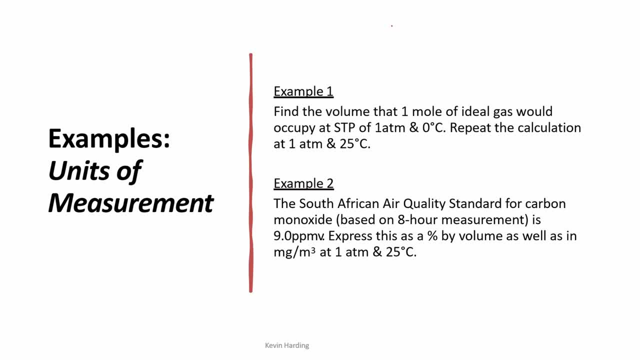 I will give you the solutions to the tuts, But probably only in two or three weeks' time, once you've actually had a chance to get them. I'm going to leave these for you to do in your own time, please, though. 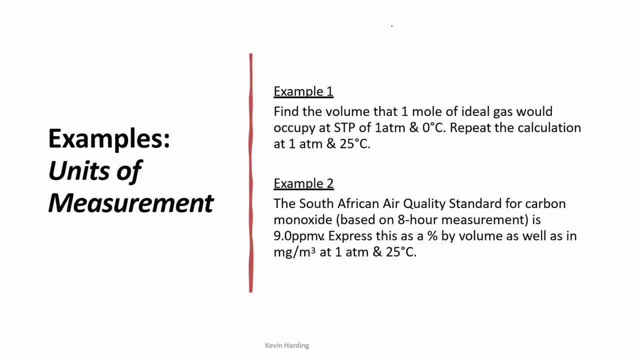 Okay, But these two and all the others in this, as that I mentioned, are probably more the type of questions that you will get from me- The next two big issues that we need. to please stop me if you need to ask any questions, or I'm going too fast, or maybe if I'm going too slowly. 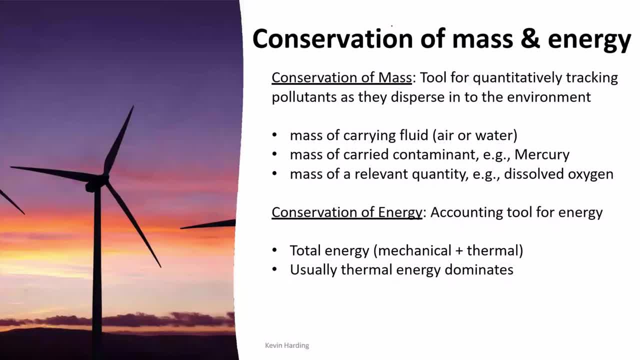 Okay, The other two big issues that we are going to focus on today is going to be the conservation of mass and energy. So, in terms of mass, the mass balance, as I said, this is what you should be well familiar with in terms of your 2021-2025 course. 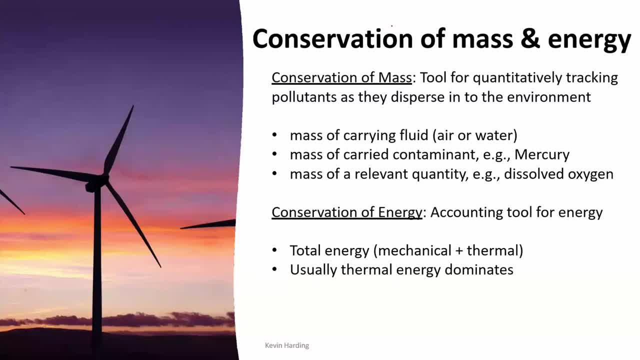 So we're saying any mass that goes in needs to equal the mass that goes out. Why this is important for this course is that you may have questions that look at a box and think the box is the or black box rather, and the word box is used in the textbook. 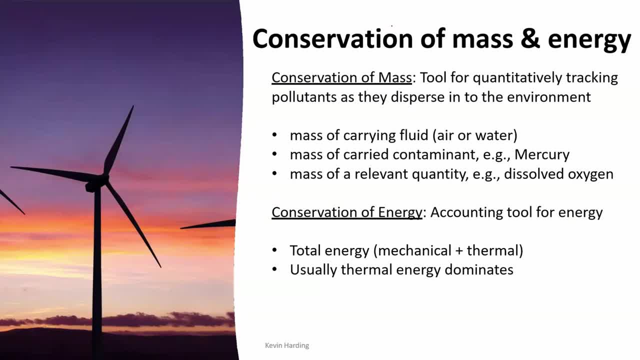 So this is only if we can get a general idea of how much mass is going to go in and out. So we're saying any mass that goes in needs to equal the mass that goes out. And then this is when we look at a fixed quantity, or sorry, a fixed volume of space above a town. 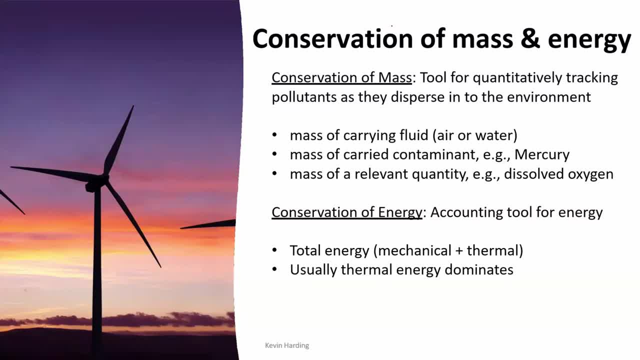 And we say that there's air going in, So obviously air needs to go out. So other examples would be something like a river water flowing down a river. If it's at steady states, we can. we can work out how much water is going in and out. 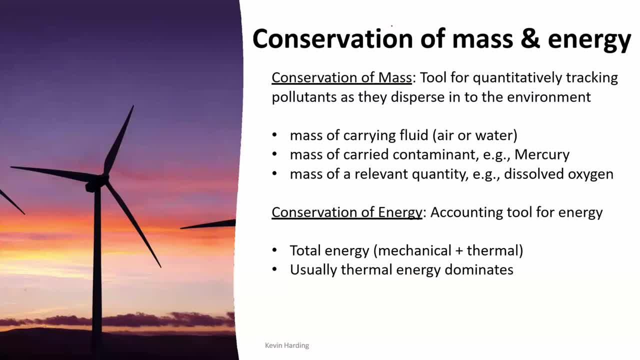 So if we know how much water is going in and out, obviously if we've given the concentration of a pollutant- so let's just say mercury- you can also calculate how much pollutant is coming into that stream. to calculate how much pollutant is coming into that stream If you have a side stream which is 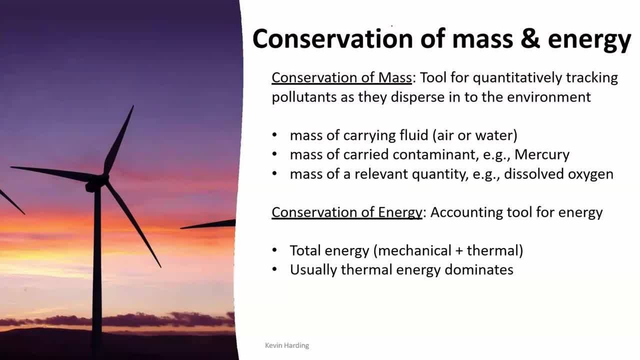 diluting it. we then know how much is coming out. So this is where I was saying that the solution to pollution is dilution. Again, a lot of companies or a lot of legislation used to say that if you have a certain volume of or certain mass of gas- but it wasn't a mass of gas- a certain concentration, 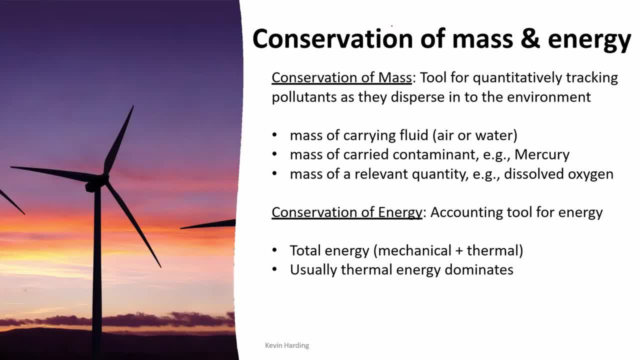 that determined whether you were within the law or not. So the easiest way to change the concentration is to just blow air as hard as possible into a side stream, so then the outlet stream is diluted. Okay, so those sort of mass balance calculations I will expect you to be. 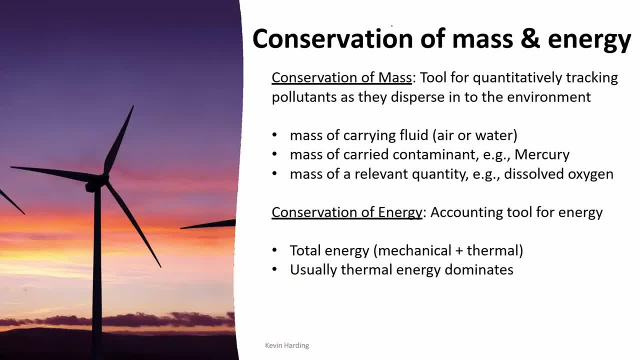 able to do, for this course, The same thing with dissolved oxygen. we could find out about dissolved oxygen In a similar way. we are also going to look at the conservation of energy. So I know that those of you that have completed this course will be able to do that. So I know that those of you 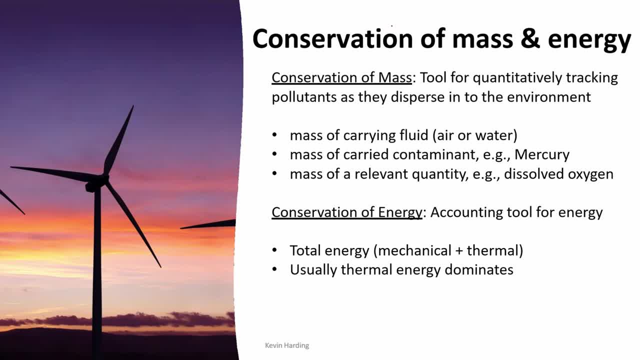 that have completed CHMT 2023 or 2028 have looked at this. Those of you that are doing thermos with metallurgy this year are probably going to look at it still. I will get back to it later. in terms of what I need you to understand for this course, though, Okay, when we talk about the conservation, 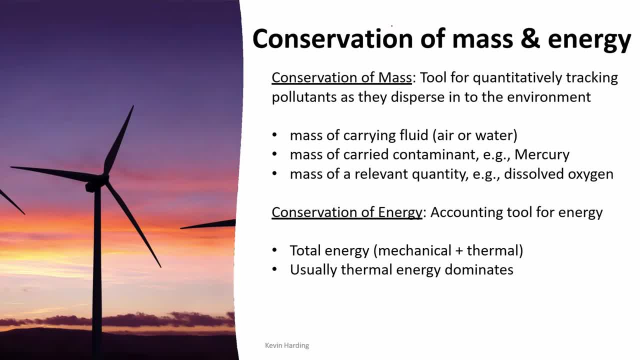 of energy. we are looking at both the thermal energy as well as mechanical energy. So it's energy from heat work. heat work and energy- the three energy types, the basic energy types, with thermal systems, as well as mechanical energy with kinetic and thermal systems. So 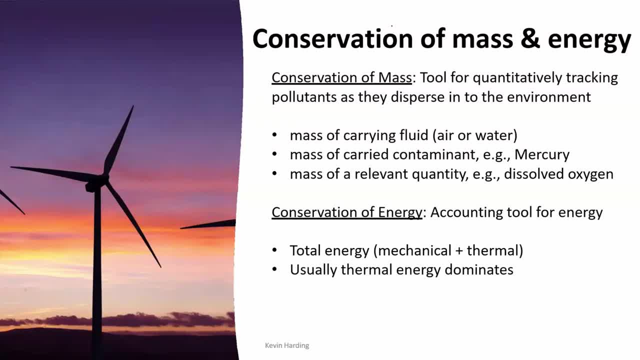 we have to look at energy that comes from an energy source, And we will talk about the energy sources as well as the energy sources for heat and potential energy. In the environmental world, it is typically the thermal energy that dominates, So we are not really going. 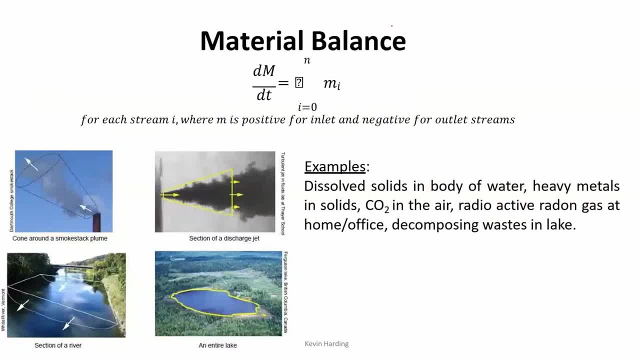 to be too worried about the mechanical energy for this. I'm still not getting interrupted, so I assume everything is okay In terms of the material balance. and I see this has gone completely funny when I play it on the slide, so let me maybe just write it on here. I am sure it was okay in the notes. So the 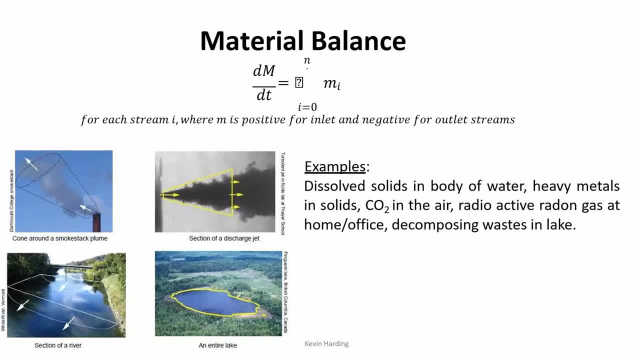 material balance or the mass balance. for those of you that don't remember, it is dm. dt is equal to the sum for i, is equal to naught to n for mi. so i'm not quite. apparently you didn't learn it in that format for 2021, but that's the format that i'm going to use, if i ever use it in this course. 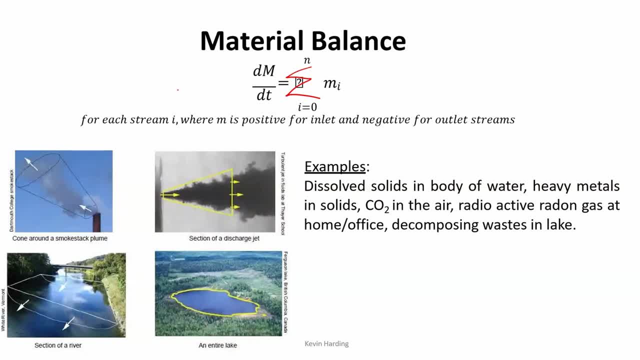 again. so that is the change in mass with a change in time. that first term, which means is referring to the unsteady state system, is what's happening inside the box. so that is anything that's happening inside. so probably you saw that as consumption and generation in your notes, so i 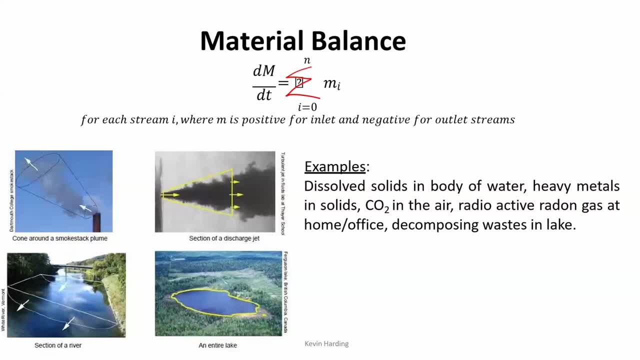 have put the links to some of my notes from- sorry- some of my videos from last year, so in particular, the derivation for this equation, the energy balance, heat transfer and some of the other things. so if you're unsure about where this comes from and you feel you need to know, please can you? 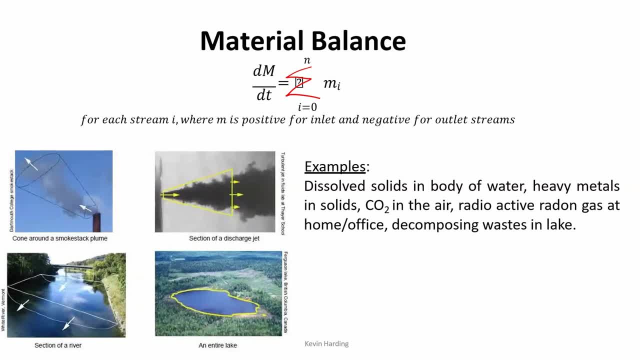 just go and have a look at that. it gives you a little bit more detail there. as a reminder, or from that derivation, rather that mi term, that is all the streams that go in and out, so it doesn't just need to be a single in and a single out. it could do as many in streams as we wanted. when m is positive, it's an inlet stream. 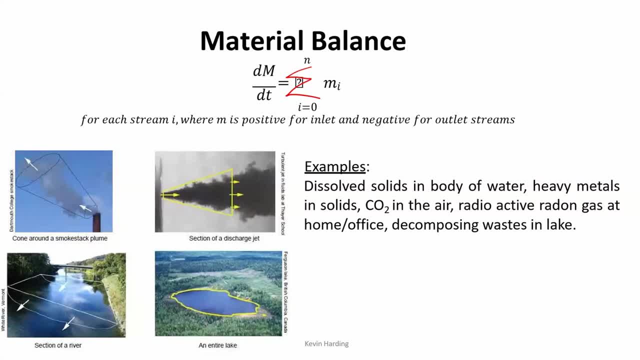 when m is negative, it's an outlet stream. okay, so some examples of that. i've got the pictures to the left there. those are probably sorry. those come straight from the previous years um notes and i'm not sure they're too useful for this. so they're just diagrams there to neaten it up. 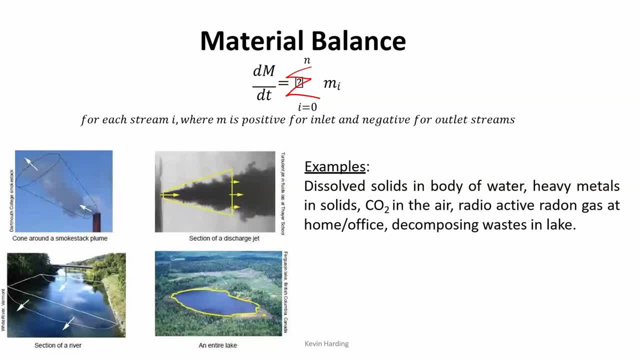 don't worry too much about those diagrams. an example where we would use this is calculating the dissolved solids in a body of water, the heavy metal co2 in air or even radioactive gas, okay, or decomposing wastes in a lake. so there are various different ways that we can look at this and i want 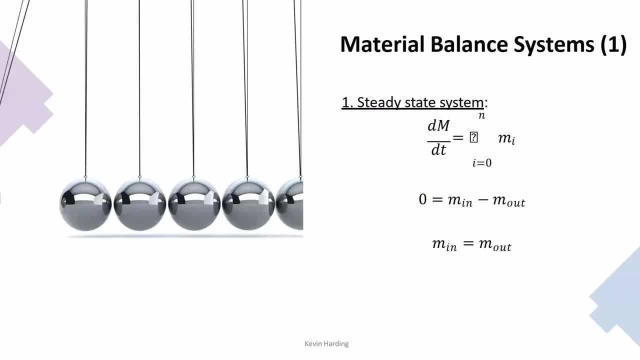 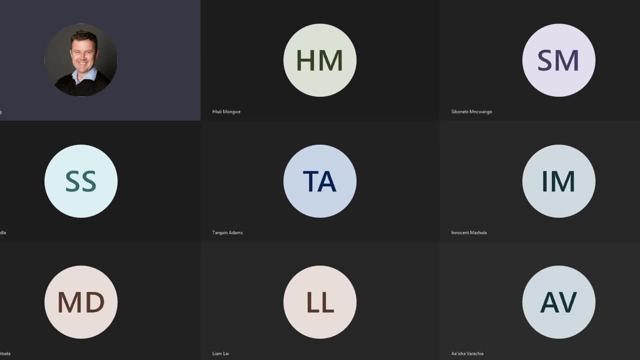 to go through some of these step by step quickly, okay, and i think let me just pause us for now and let me just go back and find out why this is not showing us the symbols, okay, so i just want to go back. i'm not quite sure why this is. uh, they've disappeared on my system as well. okay, apologies for that, i think. 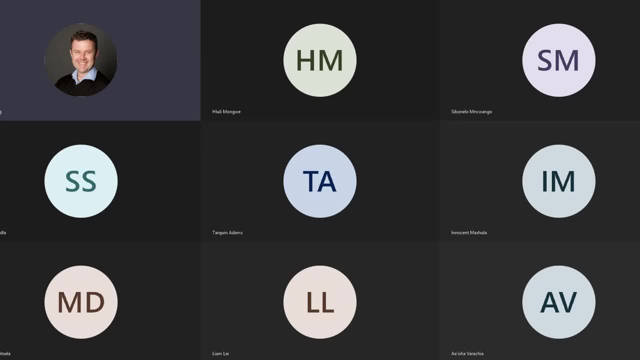 your version that you've got on that side, you probably still have the. i've got a different text or something that's not picking these up, i think. um, sorry, i just need to get this going again again. okay, so i'm not quite sure what's happened to these symbols here. i'll 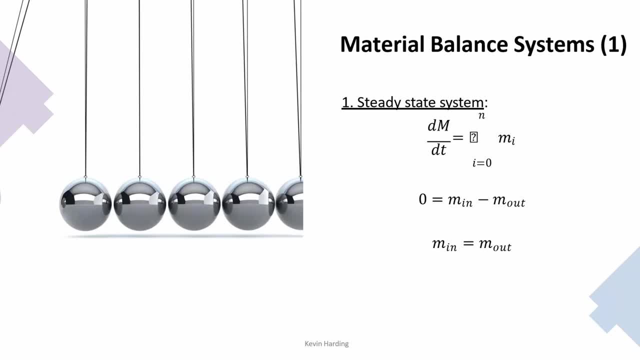 if your version. i think they are still working. okay, hang on, i've lost you guys. now just find you again, okay. so the first example on the material balance is that i want to look at is a steady state system for a steady state system. i'm trying to get the pen back. 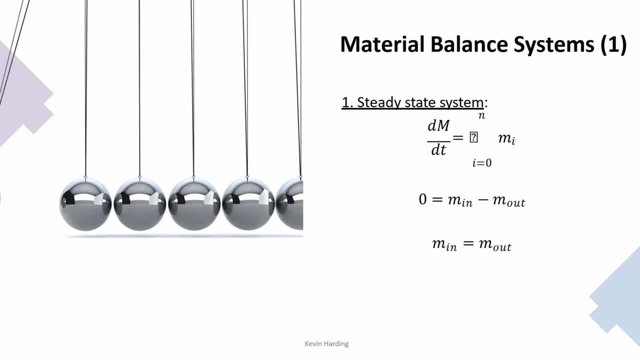 so i can fix this this as needed. oh sorry, that's not the pen, that's the highlighter. okay, so as we said, for a mass balance, the mass balance is: dmdt is equal to the sum of n of i. if it is a steady state system, that means: 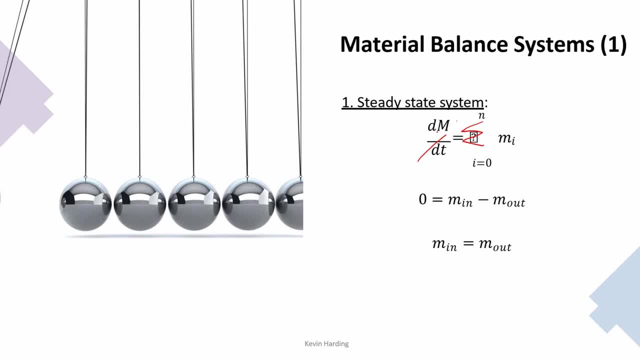 that any change in time. so steady state is defined as something changing with time. so that means the first term would be zero. if the first term is zero, we then left with. zero is equal to mass in mass out. so if we simply have a single stream- sorry, a single in and a single out, it would be mass one. 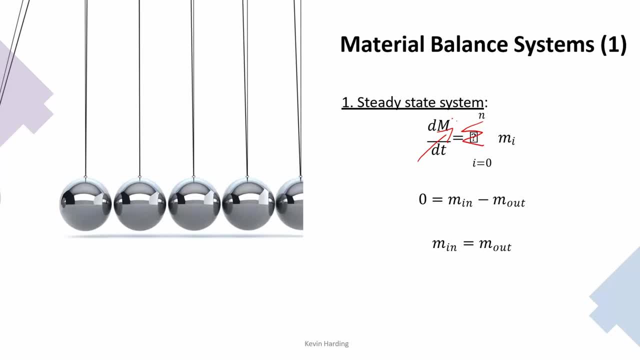 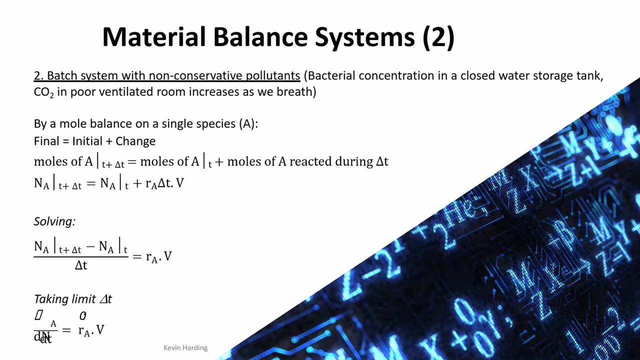 in is equal to mass one out. okay, we can then split that up into mass one plus two, plus three plus four. going in is equal to five, six, seven, eight. going out, okay, so that's the first system that i'm going to need you to understand, please. the second system: oh, and this is not even work at the bottom now. 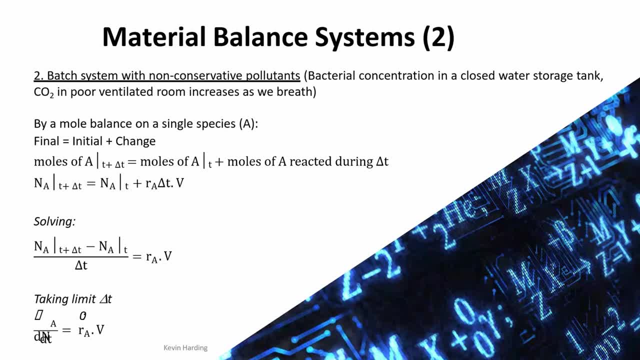 so the second system is if we have a batch system using non-conservative pollutants. so this means a reaction taking place. so if there is a reaction taking place or something is decaying, we have the example of a bacterial concentration, closed water tank or co2 in a poor ventilated room. that is. 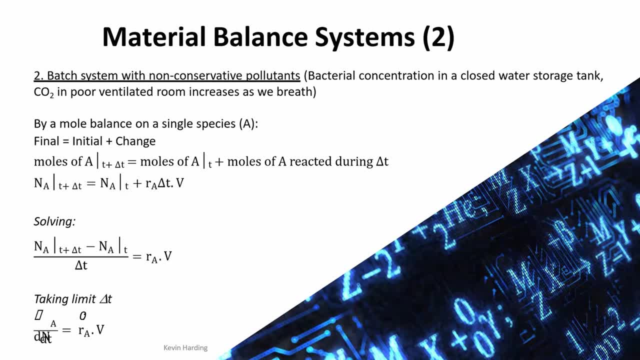 increasing. so if you and me are standing in a room with all the windows closed as we breathe, the co2 increases. so that's an example where we mean a batch system. there's no flow in, there's no flow out and the non-conservative pollutants meaning that there is a change. it's a batch system with. 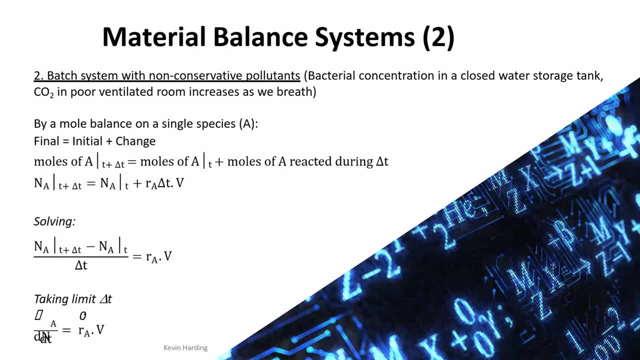 changing pollutants. so i'm putting this section up because some of you are going to need this for reactor design and you might have already taken- you're already in this- but that yellow need to know for this course. i'm just showing you so that, if you're interested, you can see. 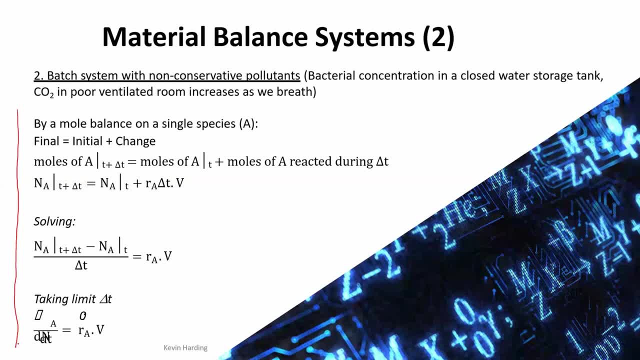 where this comes from. so if we take a batch system, we will look at that in a mole balance, because as soon as there are reactions we can't look at mass anymore, we need to look at moles, because moles react and we'll look at as the final system at time, final. 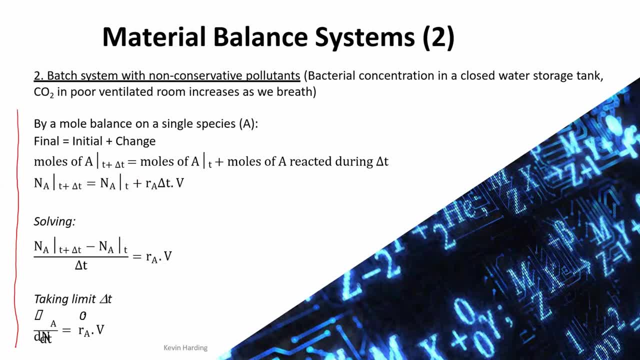 being equal to the initial time plus the change. so that is the system that we start with. so this is in terms of mole, the final moles is equal to initial moles plus the change. so writing that in more scientific notes, the moles at a of a, so we'll just call it a for now. at time t plus delta t. 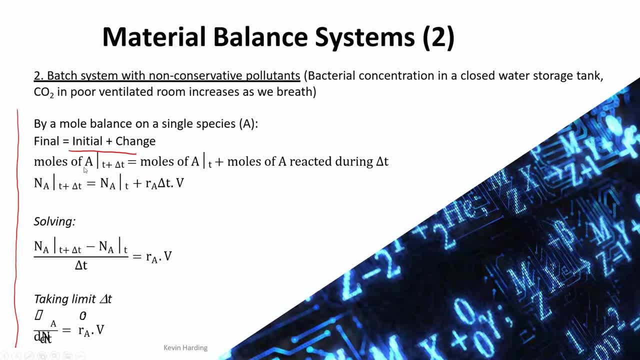 because that is the final time- is equal to the moles of a at t plus anything that reacts okay, so reaction could be increasing or decreasing. moles will just replace this in a and then we will change it to the moles of a at t plus anything that reacts okay, so reaction could be increasing or. 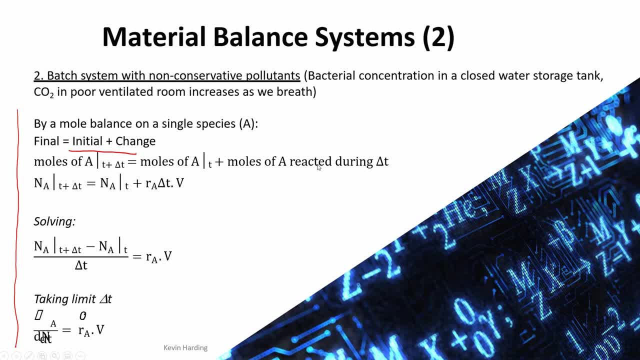 decreasing moles will just replace this in a, and then we will change it around so that n a at time, t plus t minus n a. t divided by delta- sorry- and then we'll change the moles of a reacting is the reaction rate times delta, t times volume, so then we can divide by delta. t is equal to r a on v. 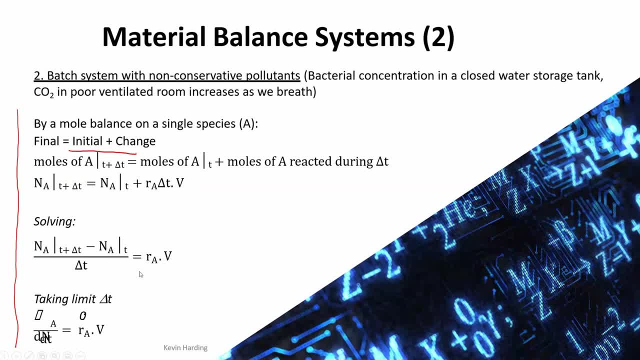 if we take the limits of delta t, as delta t tends to zero, so only more to zero. what that is is the integral of n a. sorry, i'm trying to write, it's clicking, so it's the integral and your notes should have these. i did check and i didn't see this problem last. 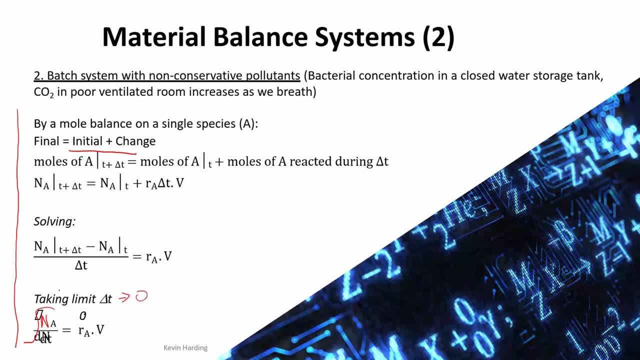 time. so it's: the integral of n a divided by dt is equal to r a v, and there's an integral on the side as well. so sorry, now there isn't an integral on that side. sorry, no, integral. okay, so we would take the integral from that. we can then simplify. oh sorry, we're. 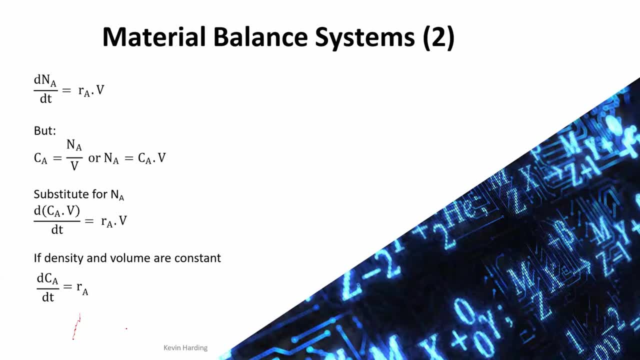 not taking it. we're taking the limits. the limit is d and a dt. i'm jumping in with a bit here, okay, so if we've got d and it's not the integral, sorry, it's the, the derivative. sorry, please interrupt me when i'm talking nonsense. some of you should have noticed. 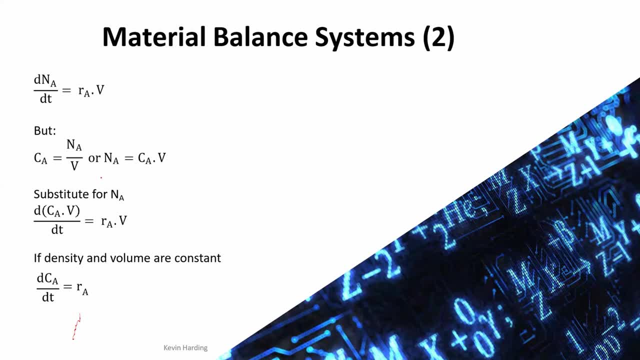 i'm talking nonsense, okay, it's just going. oh, okay, so we've now got not the integral, the derivative. taking the limit is delta. t tends to zero, gives us the derivative. so d and a, d, t is equal to r. a v is what we're left with at the bottom of the preview. should be what we're left with at the 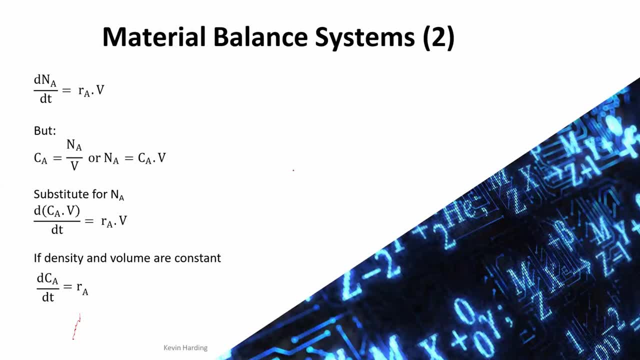 bottom of the previous page. however, we know that the number of moles, a can be rewritten as concentration. so concentration a is equal to the number of moles divided by the volume, or the na term is equal to cav. in engineering. it is very difficult to measure the concentration, but it is. 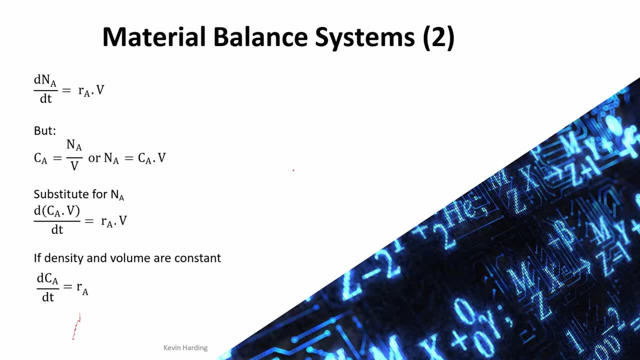 often sorry, the number of moles, but it's easier to measure a concentration. there are tools and ways of measuring concentration, but not the number of moles in a lake. so i can't if i ask you to go and work out the number of moles in a lake. 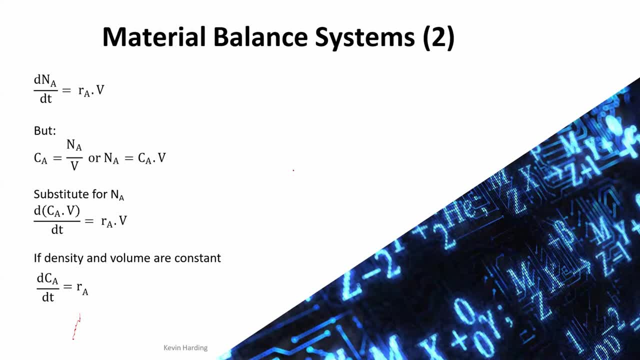 you'll take a sample of a liter, work out that concentration and then back calculate to the number of moles. so we're doing the same thing here. if i substitute the d- sorry, the na- into that equation, dca times v on dt is now equal to r a v if the density and volume are constant. 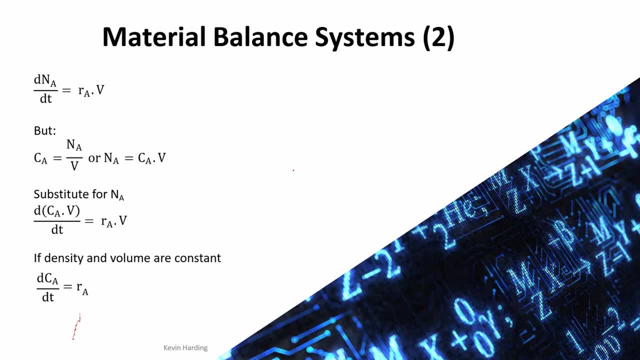 and in this course they will always be constant. we can divide through by v, so these v terms will fall away. sorry, i'm not doing too well in writing with this mouse today. they will fall away and you're left with the equation: dca, dt is r a, all of these. 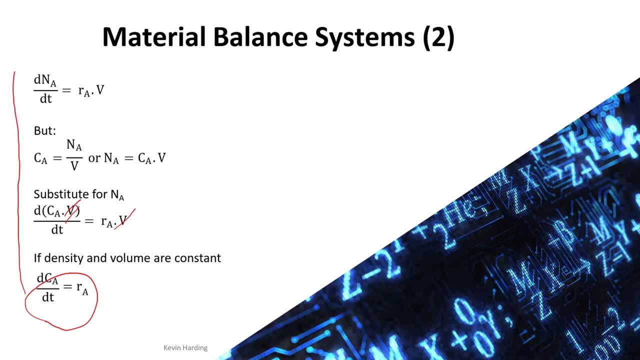 i don't need you to worry about that derivation for this course either. okay, if we take that term at the bottom. so if we just look quickly, dca dt is r a. the rate of that depends. sorry that it that r a is going to be different values for different rates, rates of reaction. so if it is a first order, 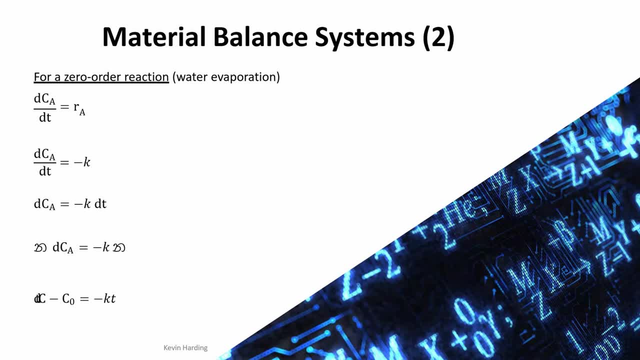 reaction- sorry, a zero order reaction. and an example here is water evaporation. dca on dt is equal to r a. we will replace r a because it's a zero reaction. that means that we just have minus k, the rate constant for this equation. separating this out, we've got dca on the left hand side is 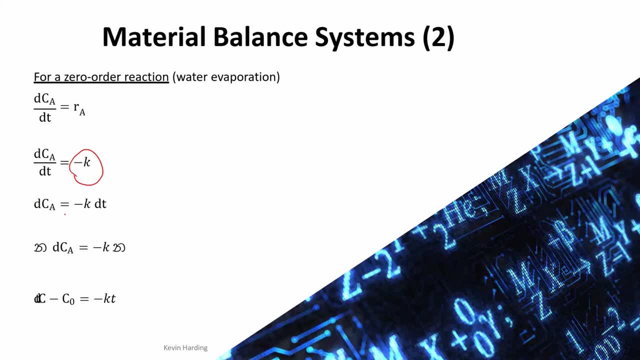 equal to kdt, and now it was where I integrate, so this would be- or maybe it's easier to put it there so you can see. so you can see- that the integral, now we integrate both sides- dca is equal to minus kdt. once I've integrated that, we'll have the concentration minus concentration naught. 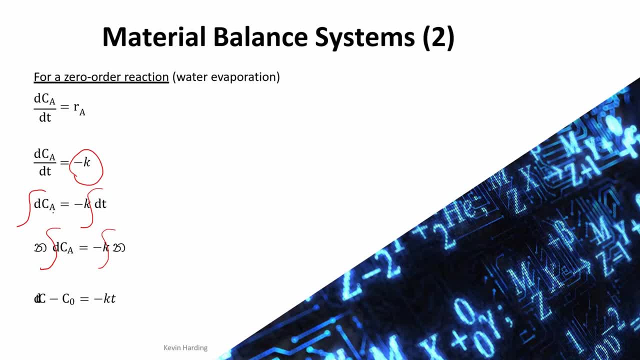 from the integral on the left hand side is equal to minus kt. okay, so let's just hide that one because it's just confusing us from the one before. I think okay for a zero order reaction, and you'll see in the examples it says for a zero order reaction. this is what comes out. 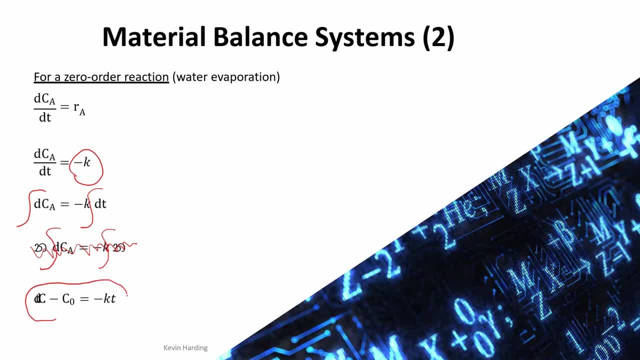 I need you to know the final equation, I don't need you to know the derivation. the exam and the test will be open book so you can have that on a piece of paper in front of you. for when I say a zero order reaction, such as water evaporating, are they us? I don't see any questions yet, so I'm assuming. 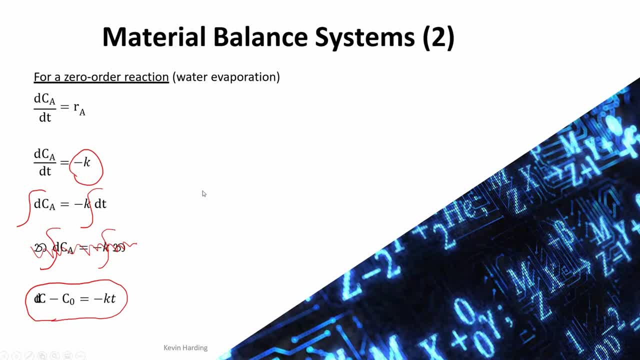 everything is still okay. in the same way, we can look at a first order reaction. so a first order reaction, oh sorry. so first reaction, we start again with: dca is equal to sorry dca, dt is equal to ra. a first order reaction from your first year chemistry, second year chemistry, you should remember. 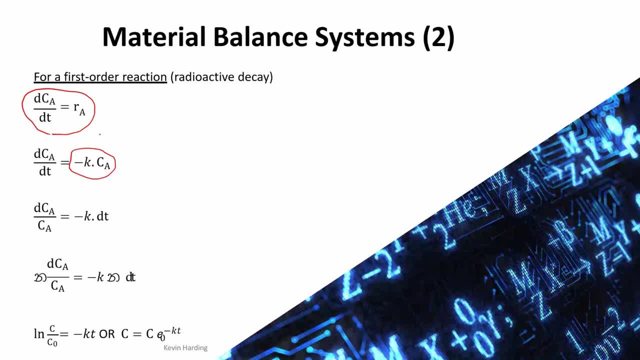 that ra would then be minus k, ca again. we can rearrange this, but we now have a ca on the right hand side, so we need to bring it down to the left. when we're looking at our separable equation- separable- and when we differentiate, integrate, rather, the k is a constant. so it'll come out. 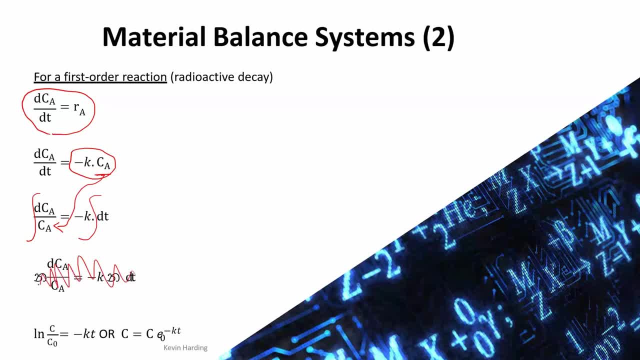 i'm going to scratch this out because my integral signs have turned into funny symbols there when we integrate, we've now got integral of ca- sorry, integral of dca on ca, so that comes out as a lin term on the bottom here and the integral on the right hand side simply comes out as a minus k. 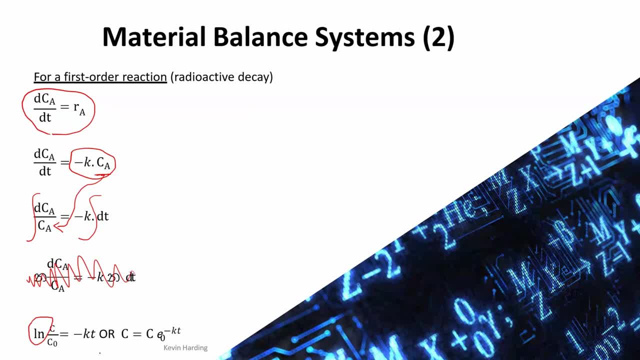 t. so we can either write that as the lin of c on of the constant concentration on the initial concentration is equal to minus kt, or get rid of that lin and change it to an e. so that should be: c is equal, c e to the power of minus k t. okay again, i don't need. 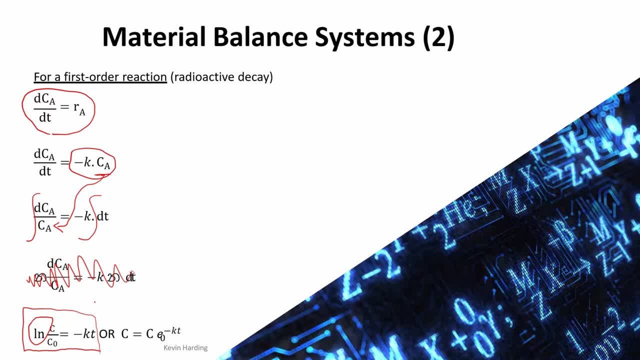 you to know the derivation, but if it's a first order reaction- and i will tell you what order it is in the exam or test- you need to know that this is the equation that you will be using for that system. third one and the last one that we are going to worry about here is if it's a third order. 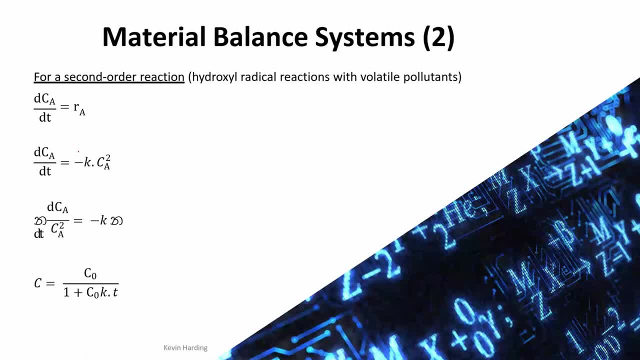 reaction. the third order reaction is going to be again: r a is going to be: r a is now equal to minus k ca squared. so that's where that term there comes from. we again. let me just cross this one out, because the integral signs have totally messed up again. 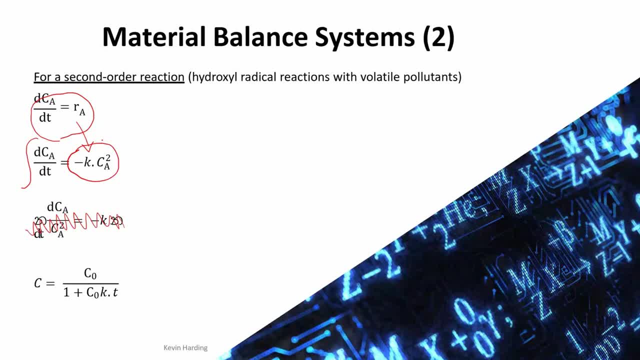 so the integral is now on that side. sorry, i've messed this up. now. integral: there. we need to bring the dt onto the left and the ca squared is going to come down to the right here as the ca squared. okay, so we're now integrating with a 1 over ca squared is equal to the minus k integral dt. 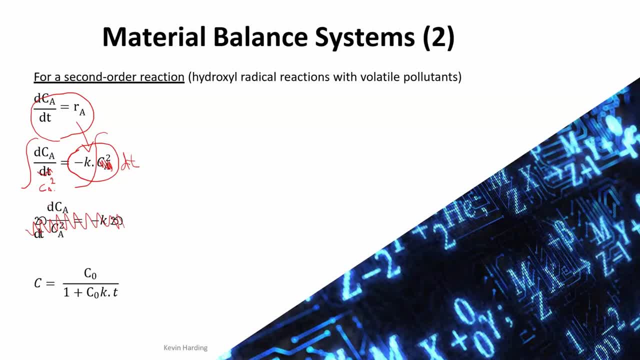 the right hand side will again be minus kt. the left hand side is a 1 over ca squared. you might want to check up on the integrating that i got from notes somewhere. it was from my notes in the previous year but that comes out as c is equal to. 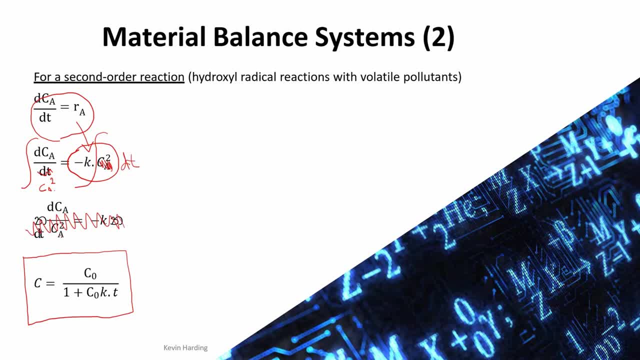 c naught divided by 1 plus c naught, kt, which i'm 99.5 sure is right. okay, so again, if it's a second order reaction, you'll get an example of hydroxyl. radical reactions of volatile pollutants are in a room or in a something. these are the code, the values calculate the concentration after a specific. 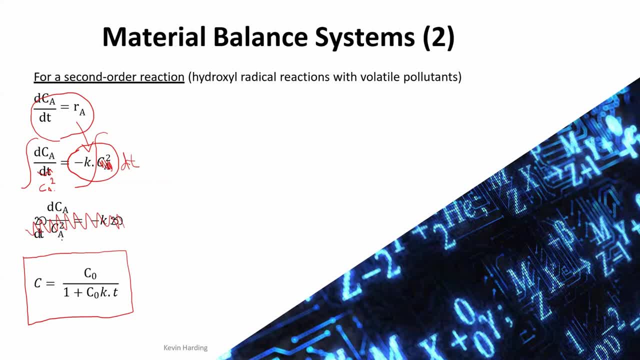 time. okay, are there any questions on that? i'm going to put you on mute for two seconds while i have a sip of water and just double check. there are no questions up to that point. okay, i'm not quite sure. there's just the word second order. that's been posted. i'm not quite. 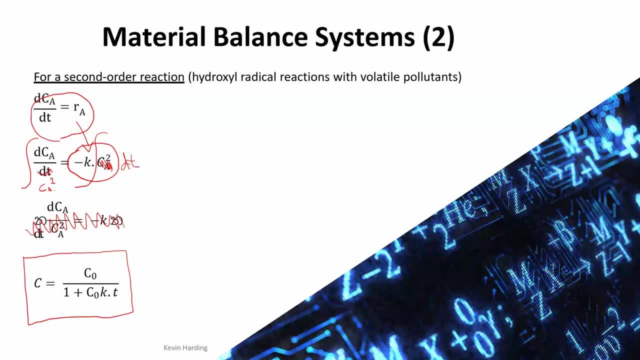 sure what you mean in gift. in the chat from big blue button i'm not seeing any other questions or anybody that wants to chip in to work to ask me for that gift. i'm waiting if you have a question from there. if there's anything other than second order, 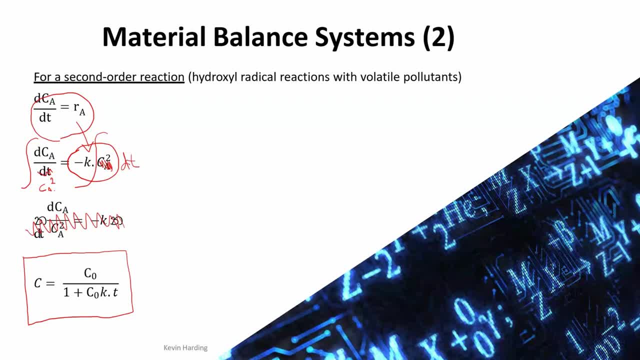 okay, so i'm going to put you on mute for a second. yeah, okay. so first of all you'll have to knee your fingers together and you'll come up and you'll find me. i'm really sorry if i'm a little off the count, okay? so in the textbook you'll 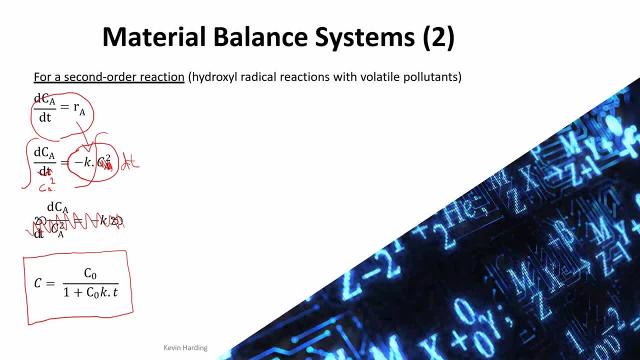 also see that when they come to examples of these. i have not done it in the tat, but i i may do it for the test or the assignment is to ask you to draw the graphs of these types of systems. okay, so draw the graph of concentration on concentration naught, one plus cokt. okay, so please make sure. 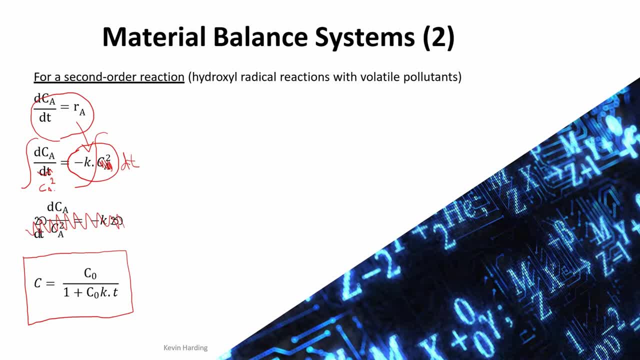 that you can draw the graphs of the concentration over time. draw a graph in a test or an exam. please make sure you draw it as accurately as possible. If you're using a pen and paper for an exam, get out your ruler and mark out as accurately as you can. 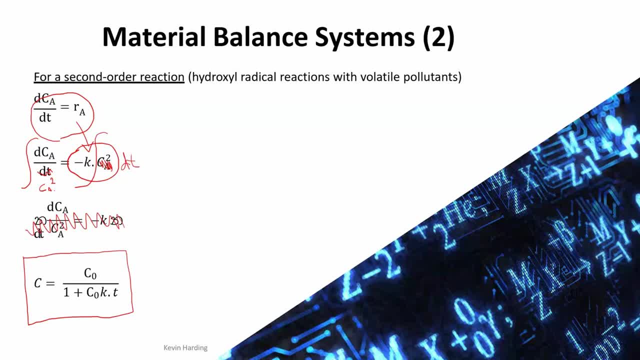 Don't just freehand it and then try, then expect to be able to read accurate numbers off that graph for me to give you the final marks for this. I realized timing was an issue, possibly for some of you, but in a test or an exam, please make sure that you do this as accurately as possible. 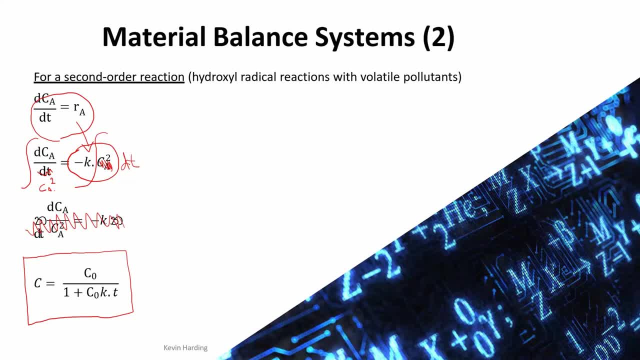 If you need to do it for a tut or an assignment, please don't forget you have a computer to draw graphs for you. Okay, is that a message coming? Sorry, I thought there was a message. Okay, so I'm assuming there are no messages. The easiest way to do these examples. so we talk about mass balance. 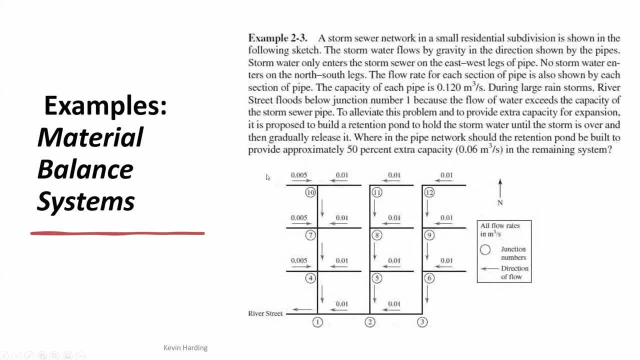 and then we go through there Again. I'm not going to go through this example now, but just to let you know that the mass balance type systems- this is a bit of a network problem. a stormwater we would probably call it in South Africa a stormwater network in a small residential. 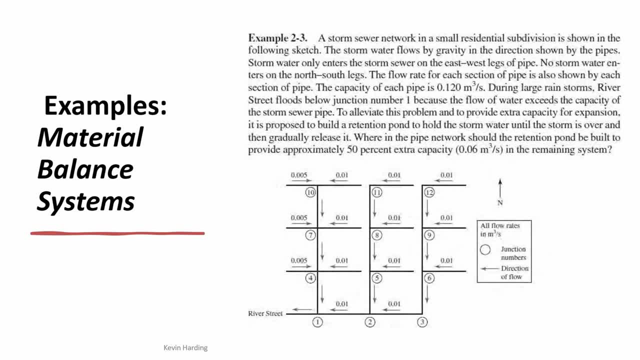 subdivision. So there you can see that You can see a network of 0.01s and 005s all converging into different things, And your job would be to calculate, be able to calculate. what are the totals at each of those points? 1,, 2,, 3,? 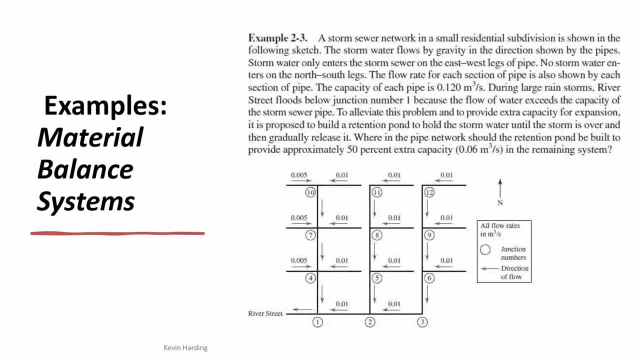 4, up to 12, and how much water goes out onto the street? I think the question is asking: So: is the piping big enough to have this sort of system? What happens if there's a flood? Is it still sufficient? Okay, that's the easy example of the straight mass balance. In is equal to out. 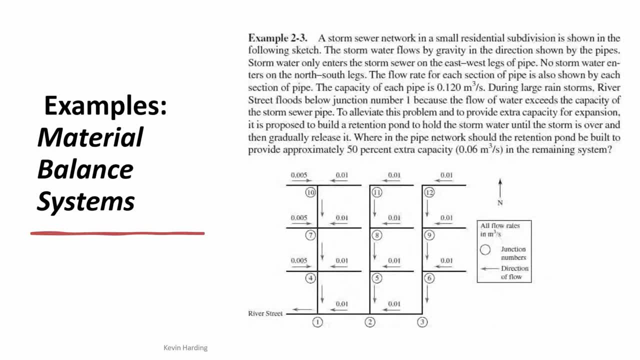 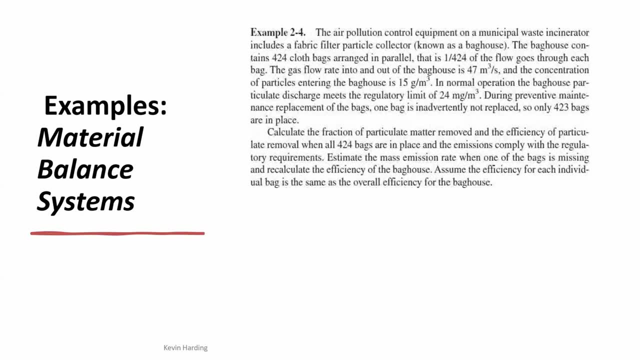 Which I think we would expect a second year in TUT1 to be able to answer. Something that it's a little bit more complicated is when we start looking at those cases of 0 order first and second. So again, I'm not going to worry about that one there. Please have a look at those sort of examples in. 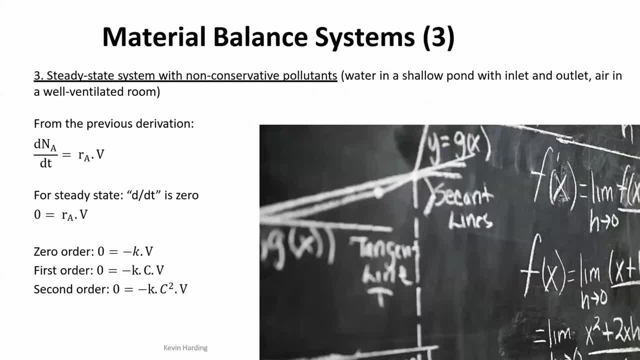 there, as well as the TUT. The third type of example that I need you to understand for this course is going to be a steady state system with non-conservative pollutants. So this is now a steady state where there is a reaction. Okay, The example here might be water in a shallow pond. So the previous example- sorry- was just an. 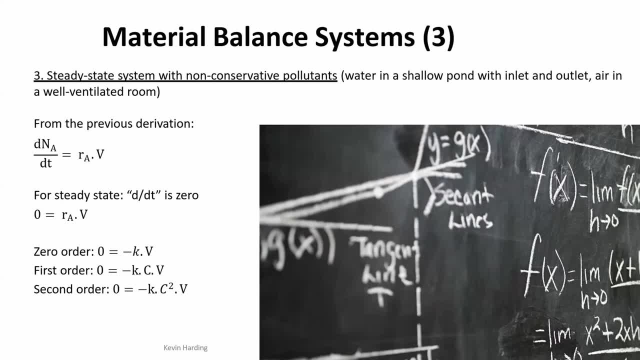 accumulation by first, second order. This one is more of a reaction. So the example here is water in a shallow pond where there is an inlet and an outlet, or air in a well-ventilated room, So we're no longer looking at you and me in a classroom where we're all breathing to increase the CO2. 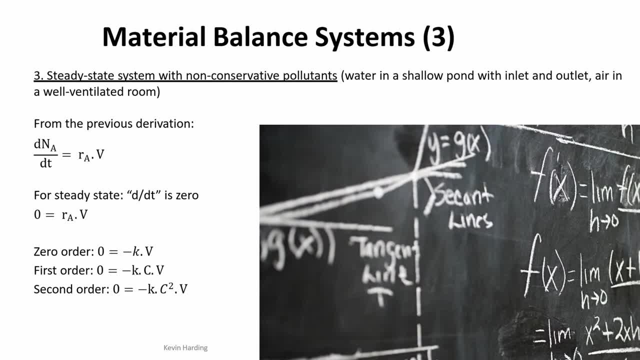 concentration. What we now do is we open up the windows. Okay, So for those of you that are looking at that are probably doing the reactors course at the moment. this is effectively starting to look at more our reactor engineering stuff. So plug flow. 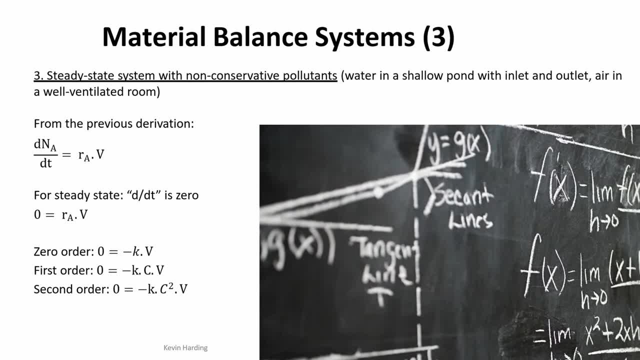 reactors. Well, you'll get in the next one, the plug flow type reactors and the CSTRs, but we'll get to that now Again for this course, anything here. So I'm skipping over a lot of the derivations, or it's not. 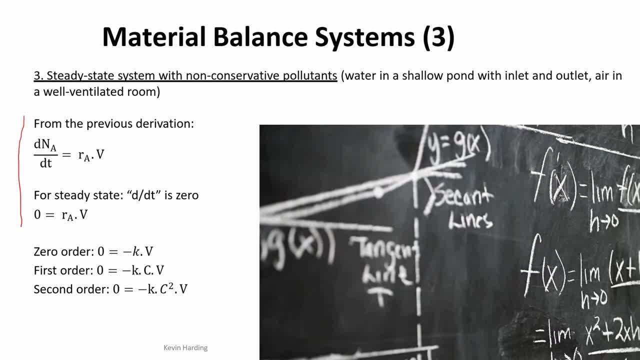 skipping over the derivation. I'm just. this is a simple derivation. rather, I don't need you to worry about the steps in between between what I need you to worry about. sorry, I've lost my mouse. I need you to know these final equations. okay, so if it's a steady state system, what steady state means is? I've said before that. 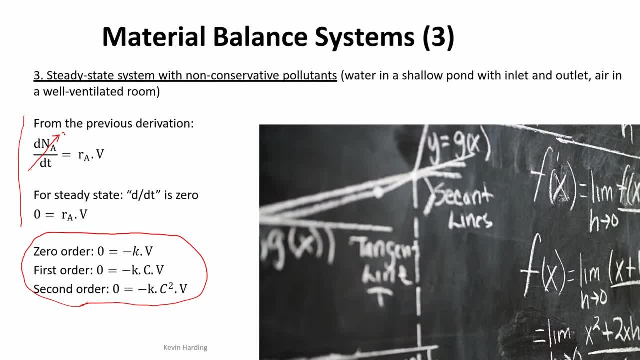 anything that has delta t falls away to be zero. so dn dt is going to fall away to be zero. sorry, that's supposed to be a zero. I don't know why my mouse is not trying to highlight it. okay, so we're saying that dn, dna dt is equal to zero. so we simply have: zero is equal to the rate. 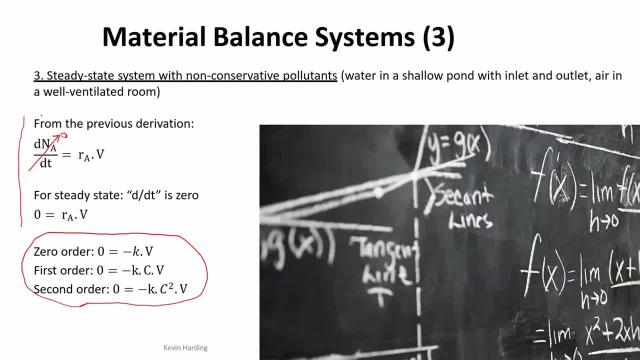 multiplied by the velocity, the velocity, the volume. if it's a zero order, first order, second order, we simply replace ra with k minus kc and minus kc squared in terms of the, the different rates for first, second, third order, and again in an exam or a test, and you'll see in the tat as well. 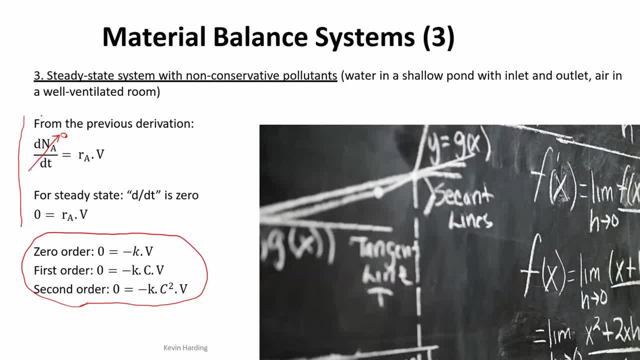 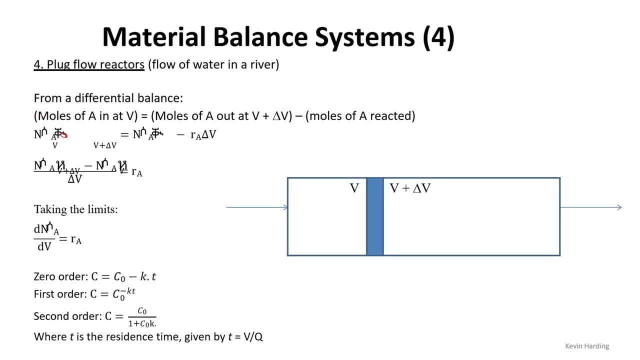 the question will go on about water in a shallow pond, something, something, something. if we assume steady state and we assume a first order reaction for the system, that's happening. what is the concentration, the volume or whatever else given a certain k value? okay, both the one and this one is looking messy and I actually, because of such a mess, I'm 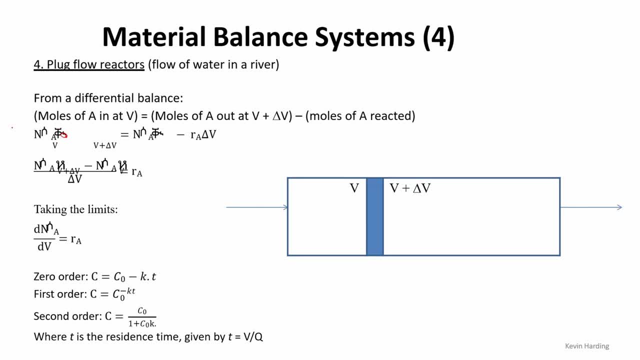 don't think I'm going to be able to neaten it up again. let me just start with the simple stuff for this course. you do not need to worry about everything up until that point. but we might have plug fluxes. so plug flow reactor is a system like we've got on the right where we've got a steady state stream. 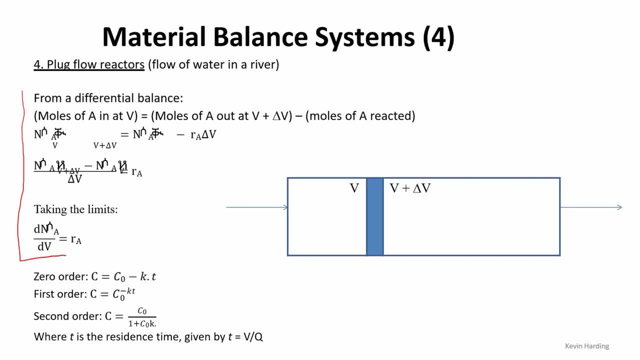 which is going in and out, and at any point along this pipe- and let me try and make a new point- so at some point along this, if I draw a section like that, the concentration at the top will be the same. sorry, I don't know what I'm doing with this mouse today. concentration at any point in 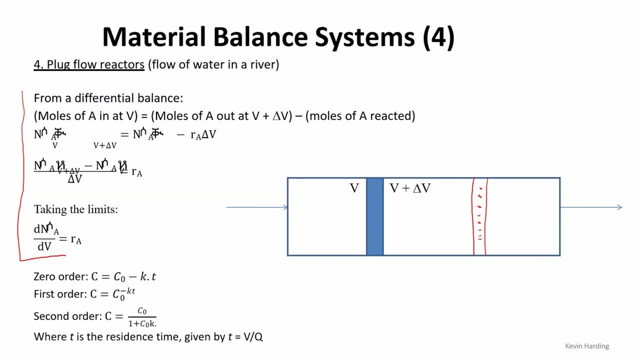 any point along that piece will be the same. okay, so concentrations on the wall are the same as a concentration at the top. so this is why it's called a plug flow reactor. the concentration flows as if it's a plug flowing through here at any given point, so it doesn't mean that there's 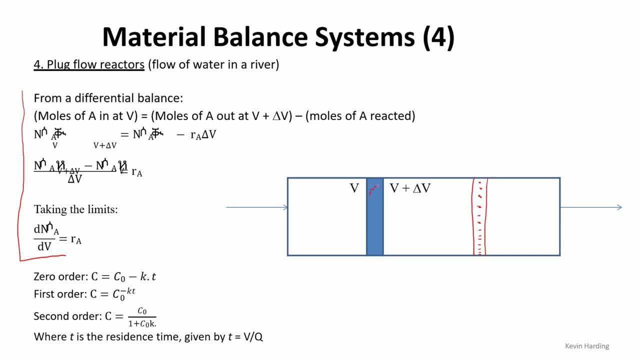 only concentration. in that plug, the blue, that I've got here, the concentration might be higher as we move from the left to the right. a concentration profile at any point along any line of the wall will be the same. so the concentration at the top will be the same as the. 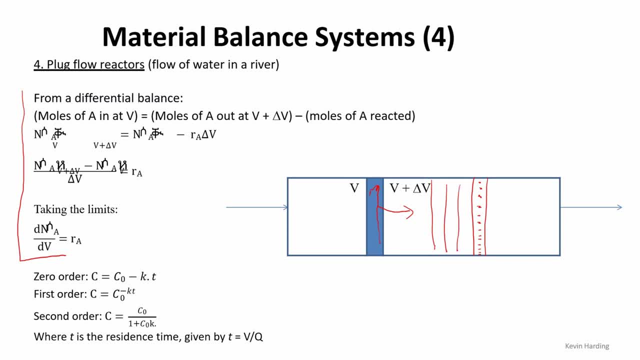 at any distance is going to be the same at the top of the bottom, but it will change from left to right. okay, so you'll notice in this diagram there is no mixing, so the mixing happens because of the flow. so this is turbulent flow that will happen in here. so the the fluid particles go all over. 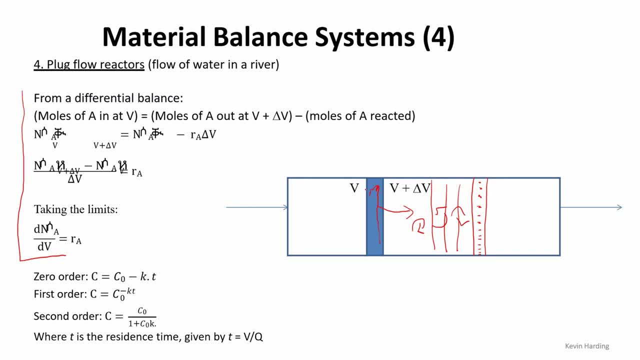 the place and because of that mixing of the particles themselves, the concentration is equal in any system, in any plug that we call it like that. okay, the derivation. so the chemical engineers- you might have seen this already- the metallurgist- I'm not sure if you see this in any of your courses this year, sorry, I just know the chemical engineering. 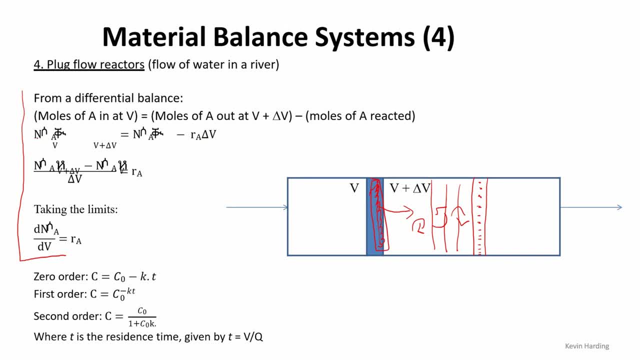 curriculum better than the metallurgy one. that's why I know where it comes. we can again look at that blue section and look at this in terms of a mole balance. so the moles of a, of a at v- so that's the left hand side- is equal to the moles of a out of that portion, v plus minus or plus anything. 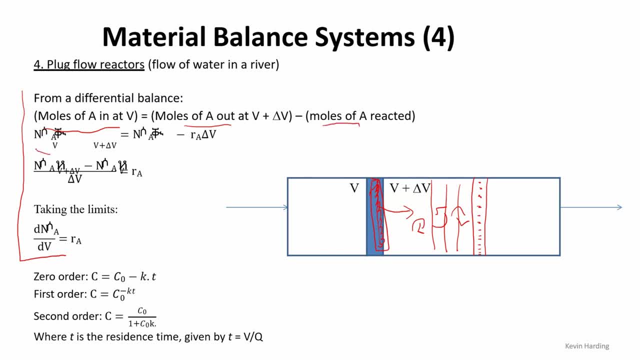 that's reacted. okay, so that's the derivation, so the chemical engineers, you might have seen this already. so what I've done here is I've changed that to the number of moles in a and then it's again at v plus delta. v is equal to the number of moles of a at v plus delta v minus those that react. so it's 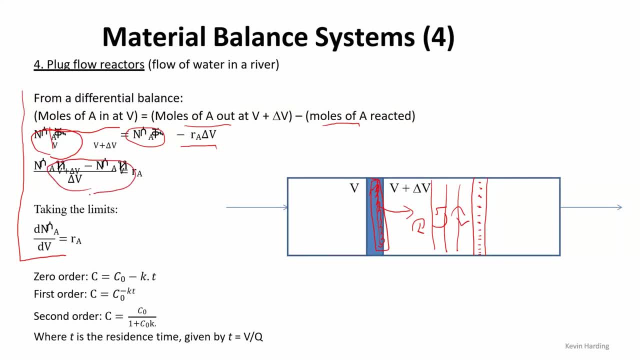 r a delta v, if I again rearrange. so all the n? a's are on the left hand side divided by v. take the limits, as delta v tends to zero. sorry, that's a delta v tends to zero. we can then have the change in number of moles divided by dv. 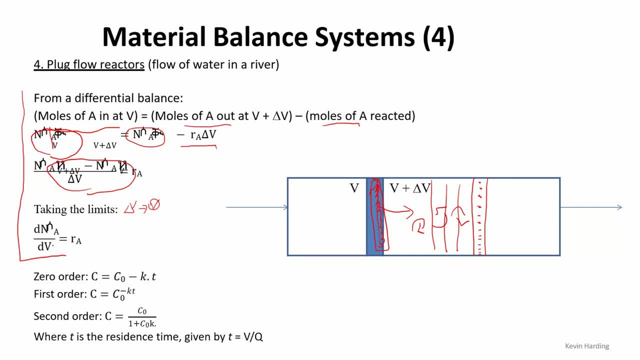 is equal to r a. okay, so that's, that one's actually fairly neat. we can just get rid of that, that squiggle there. so d and a change in number of moles with a change in volume is equal to the rate of reaction r a. what I need you to know is if we then solve that for the rates of reaction. 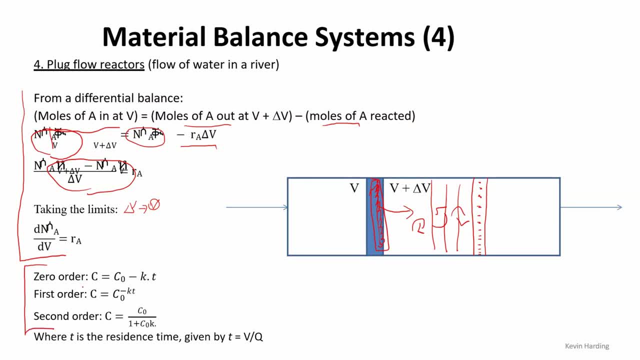 you end up with the equations: the concentration is equal to the concentration naught minus k t. c is equal to c naught to the power of k t. and the second order reaction will be concentrations equal to c naught divided by one plus c o k. I'm sure they should. let me just double check that. I think. 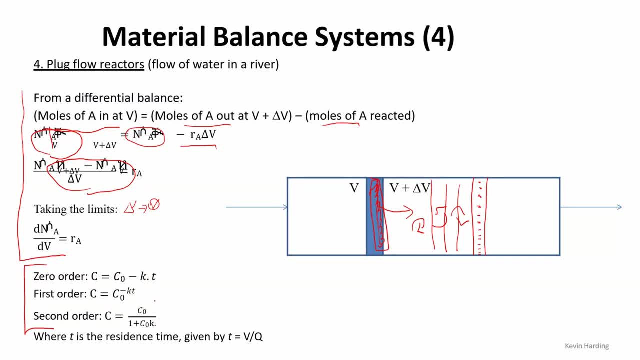 there should be a t in there as well, so please just come back and check those equations later. the thing here is that I've skipped a step in the derivation that you need to don't need to worry about. this is not t, this is not time, this is a residence time, so it's supposed to be not. 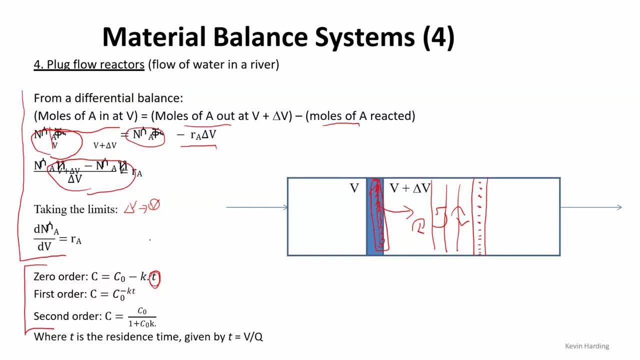 italicized t, which I think it's like it is, but I think everything's italicized, so it doesn't really note. you can't tell it's italicized, so it's not italicized, so it's not italicized. so it's actually simple because it's not so difficult, as we are not used to it, you know. so it's a. 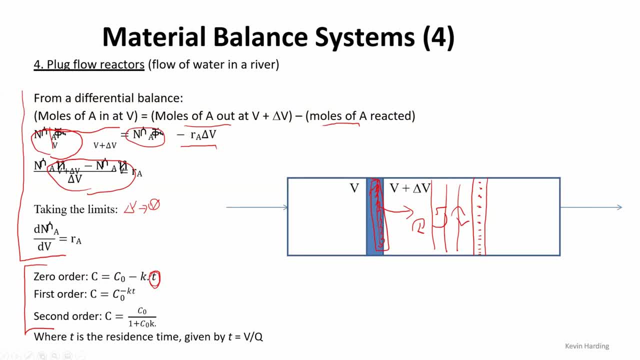 little bit more complicated than it is and it's very simple, but I'm going to pick it up there, where the residence time is given as the volume v divided by q. so I've written it down to the bottom here. so v is the volume and q is the volumetric flow rate, so the volumetric flow. 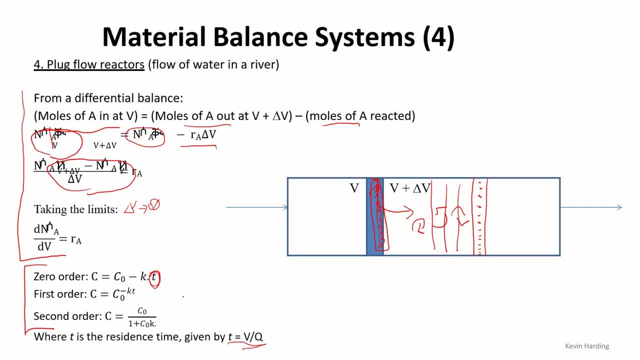 rate has a per second in it, so you can see that that's where the time comes in here, the concept of a residence time. okay, so there are examples, and you could get an example again of water flows in a river. we can model this as a plug flow reactor. 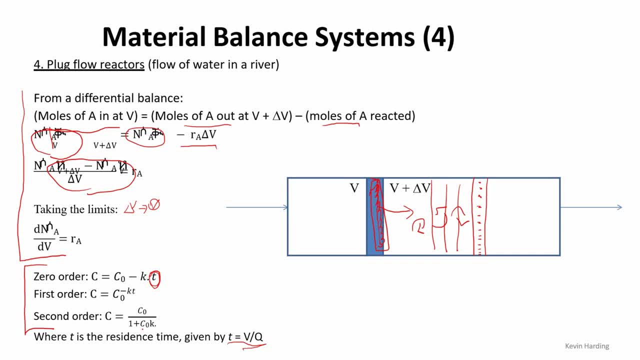 order: sorry at a zero order. first order. second order: calculate the residence time or calculate the volumetric flow rate. so if you ask to do that, you will work out the residence time and then substitute it back into the residence time equal v on q and then you can solve the volume. 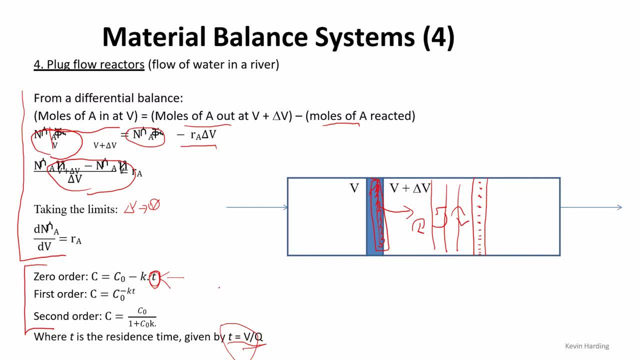 or the volumetric flow rate. however, the question wants to ask it to you. i'm getting very little interaction today, so i'm just assuming everyone is okay with this, but it's as simple as anything today. please get the yes, no, hello somebody that i'm actually. i'm sure somebody would have. 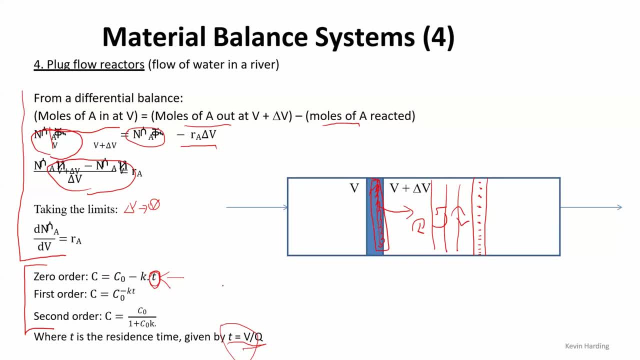 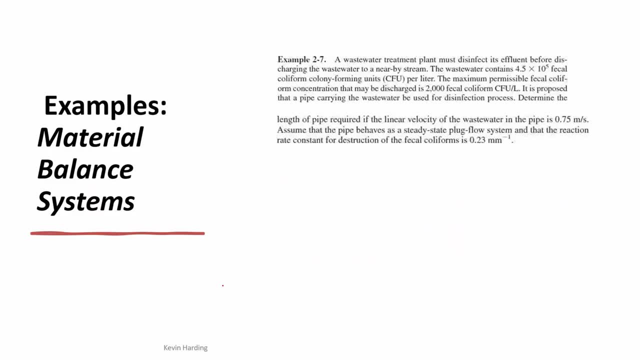 sent me an email by now to tell me that i'm not online. if i'm not online, okay, so we're all happy with that. the example of that. as i say, i'm not going to go through this. oh sorry, big blue button. i see there's a bit of a lag on your screen, so just tell me if i'm going. 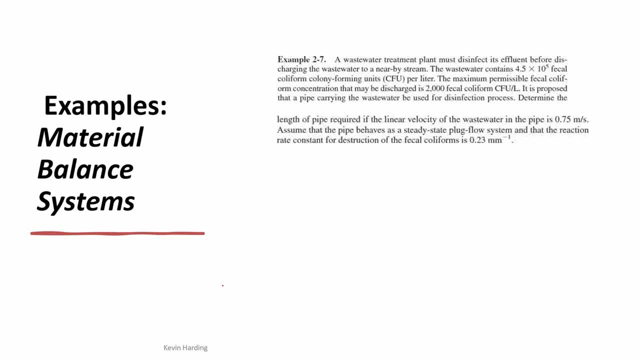 too fast or not and skipping through some of the stuff. the example again: we could have a wastewater treatment plant and again, just to show you here you'll see the sorry, i'm pressing buttons accidentally, okay, so as i say in an example, you'll get some word problem, you'll get all the. 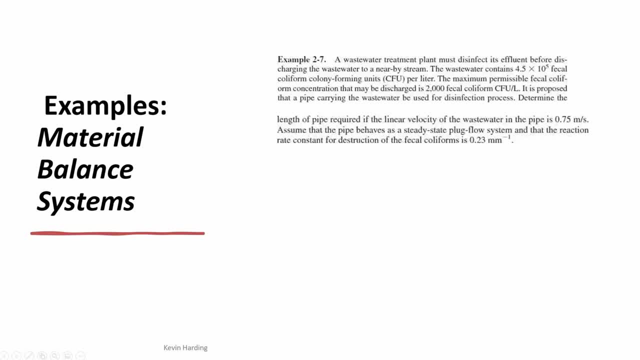 ah, sorry, you'll get all the numbers. i accidentally click this off here so you'll get a question with all the numbers. i'm not. i don't know why this is not there we go. you'll get all the numbers randomly in here: 0.45, 2000 and various other. 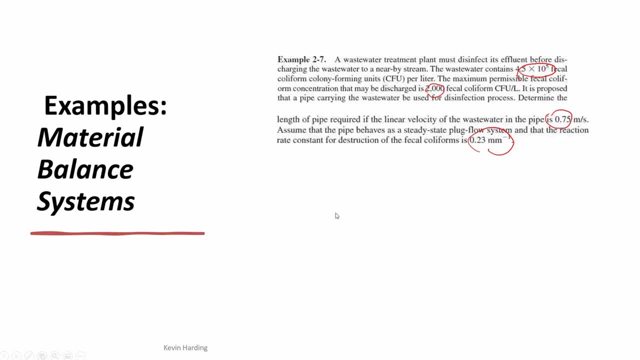 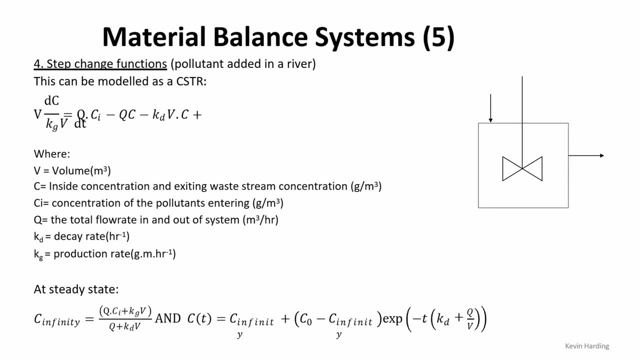 numbers which you will then need to plug into that equation to solve for whatever's being asked. okay, the next one on material balance. material balance- i've got it down- is the fifth thing that you need to know is a step change. so by a step change, we are going to model this as a cstr, a cstr. 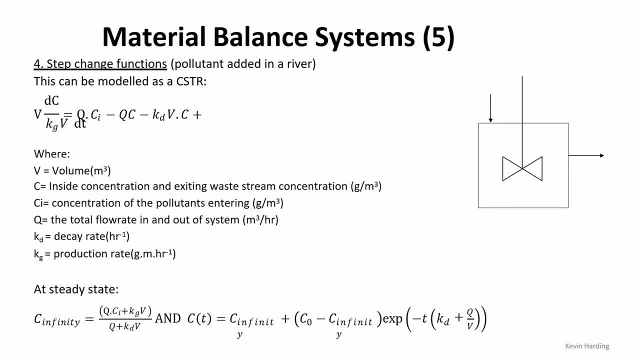 is a continuous stirred tank reactor, so a continuous stirred tank reactor. i've got a diagram there on the right and i think this one. i'm going to ask you to go and see the equation on your own, because this is a total mess on this. sorry, a continuous stirred tank reactor is going to have an inlet stream and 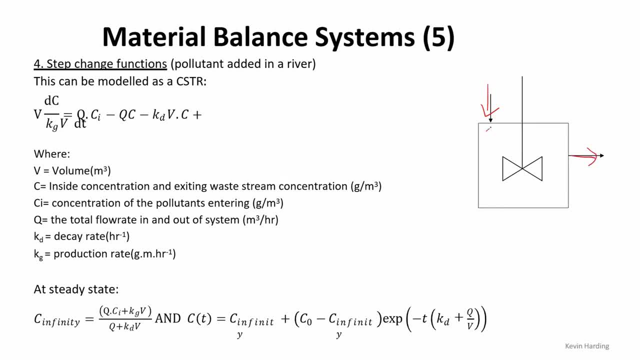 it's going to have an outlet stream. so the reaction happens in this tank and, as the name suggests, it's continually stirred. and what we assume with that continually stirred system is that the concentration inside is equal at any point. so anywhere within this entire tank the concentration is the same. so it's 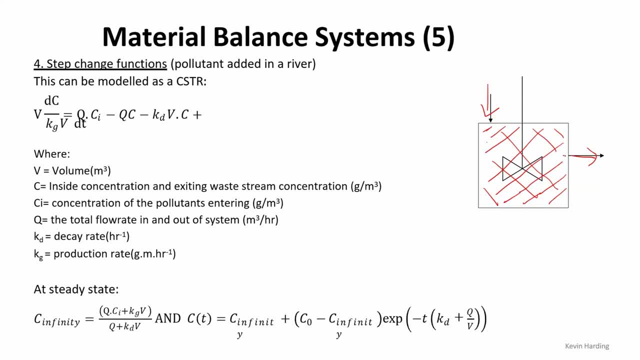 an instantaneous. everything is the same concentration and it means that whatever's coming out of this reactor has the same concentration. so this concentration, the concentration that you can see there, is equal to the concentration out. let's just call it out. so: concentration inside, that c has disappeared inside, is equal to the concentration out. 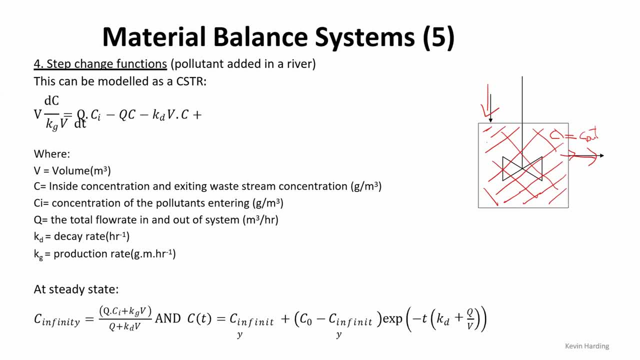 so you can again look at this and model this as a mass balance. so from a mass balance point of view, we start with the number of moles, so the number of moles coming in, there's a reaction, they're out and we end up with an equation and i can't even make out what this is supposed to. 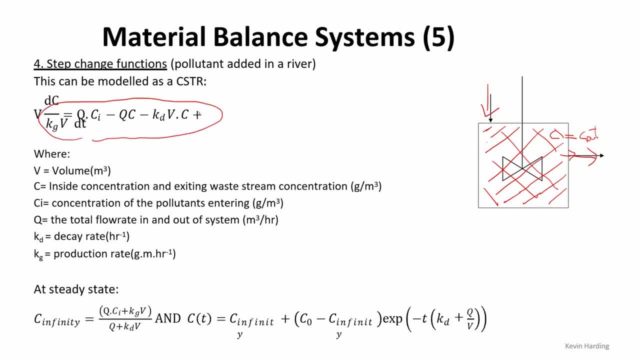 say we end up with this equation that should be here. please can you go and look at the notes yourself? that's just going to confuse me. i'm not crossing it out, i'm just sort of trying to not get my head confused by looking at it. please go look at that equation. i've not included the 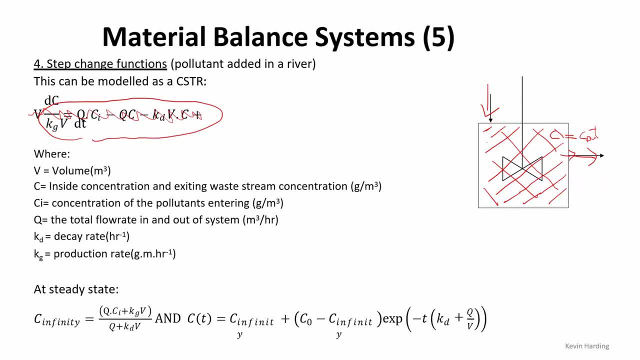 derivation here. all i need you to know is that that is the final equation somewhere in there. okay, that version that i've given you in the notes. there are two parts in this equation that you might not have come come across before, even if you have seen this equation before. this equation has been. 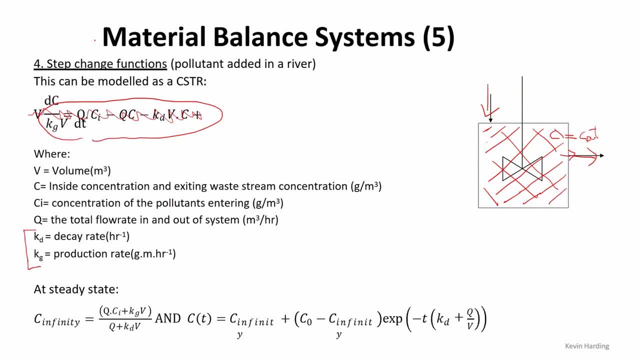 split into two, so the first, or sorry, the second. the rate equation has been split in, okay, so let me go back and do that again, again. so please can i ask you to go and look at the equation in the top here? so let me maybe rub that out. so the only reason i rubbed out, because my head is trying to think of one thing and i'm 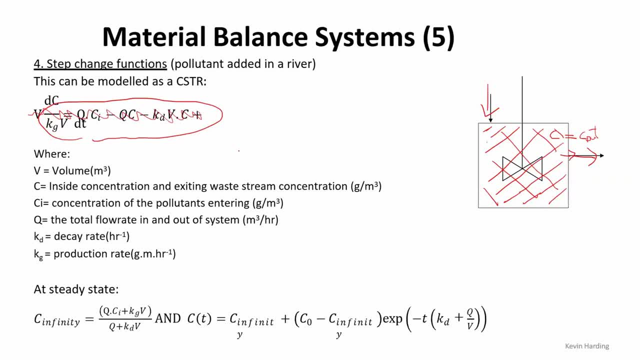 doing another thing. okay, so please go and have a look at this equation. let me just get it back like that to find the proper form. some of you may have already seen the equation for a cstr, the equation for cstr in reactor engineering or one of your other courses already. this equation in front of me. 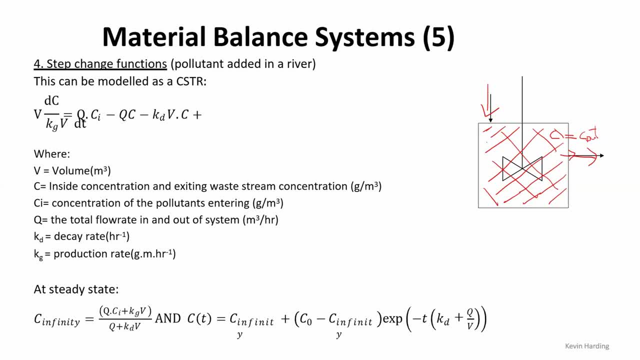 is possibly going to look slightly different to the one that you've seen before. the reason for that is that there are two rate constants. there are two rate constants. in this one there's a kd value- sorry, there's a kd value hidden in there- and there's a k g hit value somewhere in that equation. 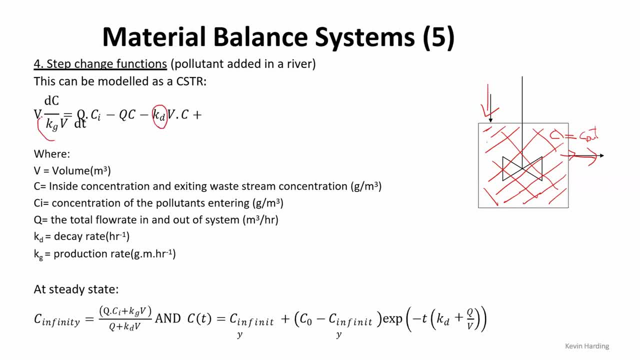 as i say, please go look at the correct form of this. it's muddled up on the screen for some reason. the d value is the rate equation when there is a decay. so the decay could be some, some pollutant that is just decaying over time, bacterial mechanism happening there. that is then. 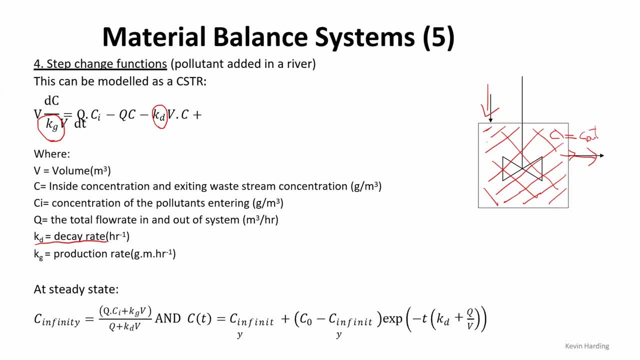 easing away at something. so that is a decay rate. it's a reduction in in whatever the pollutant is, there may also be a production rate. there is a chemical reaction happening and something is increasing. it is not always going to be the case that you have both kd. 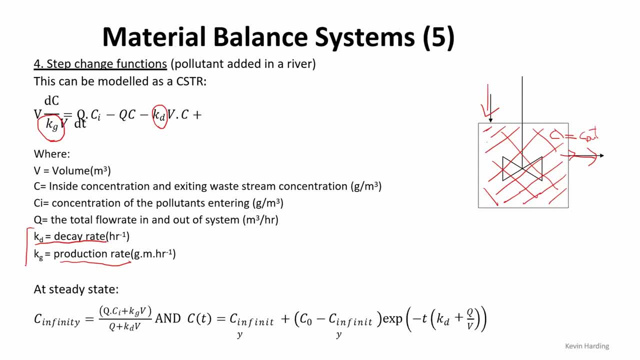 and kg in your equation. so often you will only have one. so when you have your questions that come through from your test or your exam, please just make sure that you know which one is decay, which one's decreasing and which one's producing coming up. so obviously, whichever one is not around. 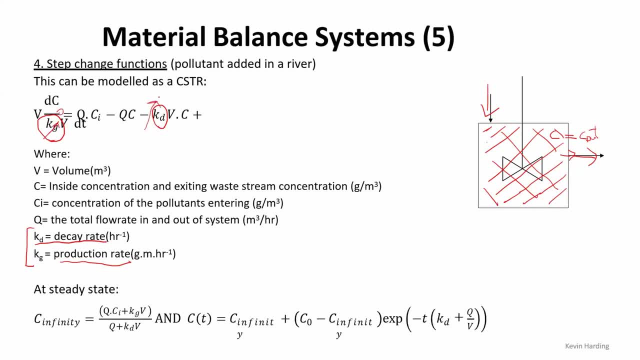 will fall away to be zero. okay, so that's quite skew. so just play it, please. you'll probably. there are very few cases when both will come into play. once you've decreased, once you've cut it out- either the kg or the kd, the equation will now look similar to the way that some of you have. 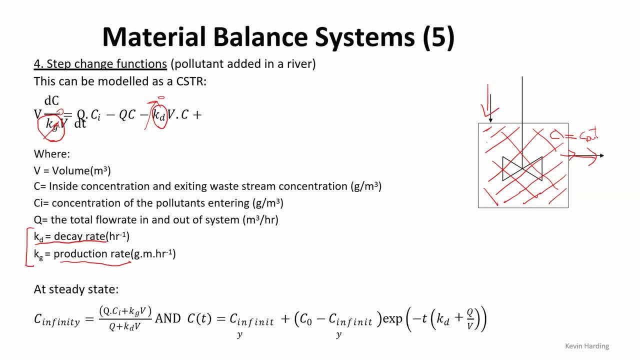 possibly seen it before? okay, did that clarify it? was i clear enough? the? was the line better this time when i was explaining it? okay, the other thing that we can do- and again i'm not going to ask you to worry about the derivation- is that if we are at steady state, we can reorganize that equation. that 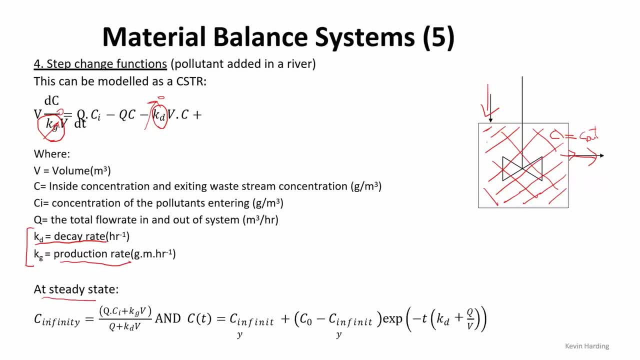 you need to go and just double check up on to calculate what is the concentration at infinity. so that's in terms of time, and you can rearrange that original equation to be like that, or if we're just looking at a concentration at a specific time. so what is the concentration after two minutes? 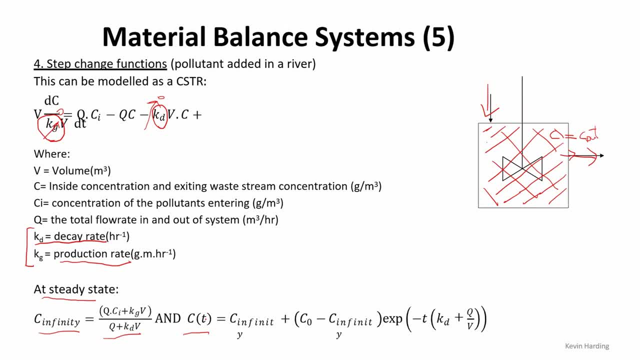 five minutes, ten minutes. you'd have to convert that into seconds. just please keep an eye out, as always, for units. make sure that your units are consistent. i see in this equation i've used it as per hour. if i'm using per hour, all of these things need to be as per hour. 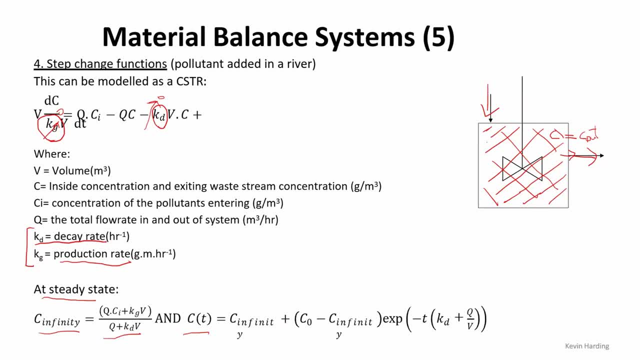 it's probably more common to have these type of things- systems as per second. so if you need to work out the concentration at 300 seconds, you can then use this equation to work that out. okay, and it's probably a little bit more clearer in the notes when i've got the spacing. 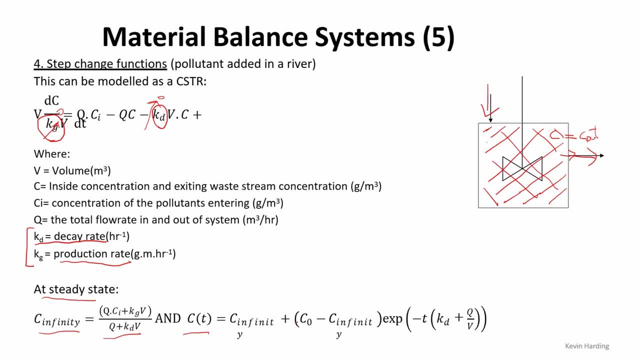 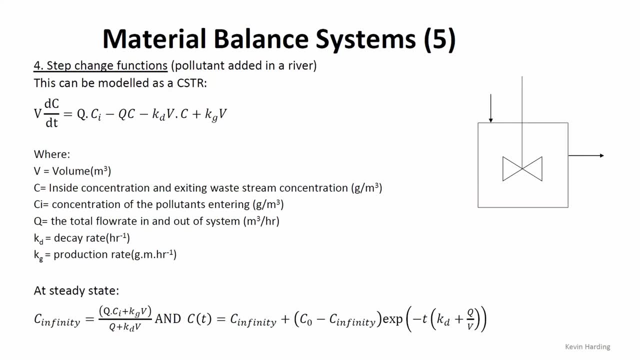 right on this one as well, okay, okay. so while we were on the break, liam was asking if the units balance, so please just double check. if so, in all of these equations that you've got and i've put, i've moved over to the um presentation that you've got, so all the equations are now sitting correctly. 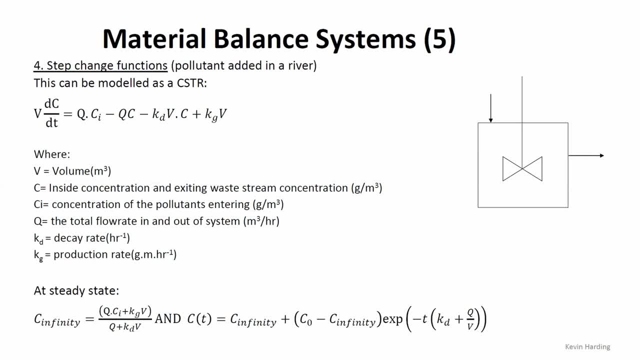 so you're just gonna have to work through the sum of all those equations and then add them in your formula. so, as we were looking here at the end of the slide, you're going to want to compare all of the equations and decide whether it's going to be consistent or not, because that's what it's going. 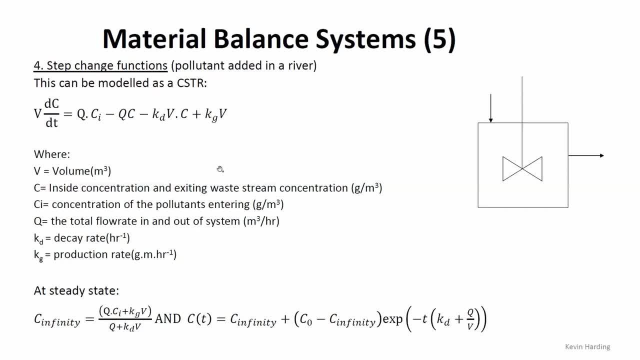 to look like now, so i'm going to give you a few tips about that to see if you could figure it out yourself. units aren't balancing, so we can just check the equation. So maybe there was a slight typo in the equations. Okay, So, as we said, we stopped. We've been doing all of the different material balance. 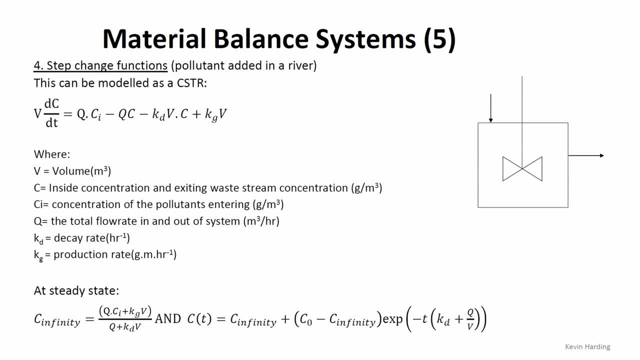 scenarios that you might get in this course. Again, I do not need you to know any of the derivations And, sorry, I can't draw Now that I've moved on to this version of the PDF. I can't draw in this. So the final equations, if I need to ask you, the concentration at infinity, the 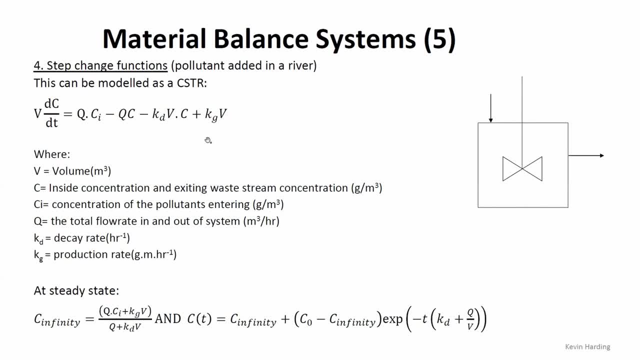 concentration at a specific time, or if I need you to just work out the concentration or something else. I will only ask you for those, for you to plug the numbers into the equations. I'm not going to ask you for any sorts of derivations anywhere in any of these things that we are doing. 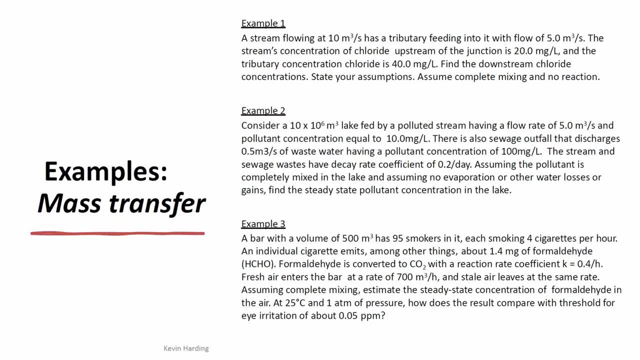 Okay, The last one, on this side of things, is going to be the examples that we might have on mass balance. So these examples here again. I'm not going to worry about doing any of them now, and I'll probably. I may or may not give you the examples, the answers to this, but these are good examples for 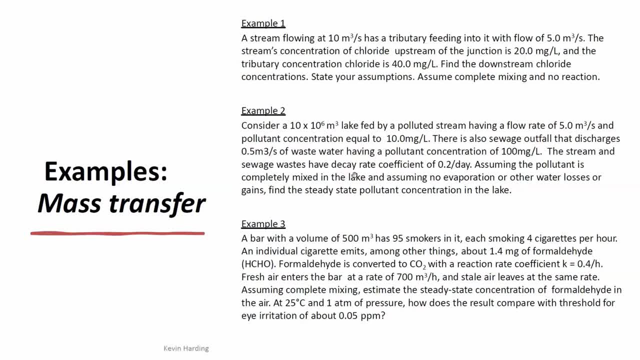 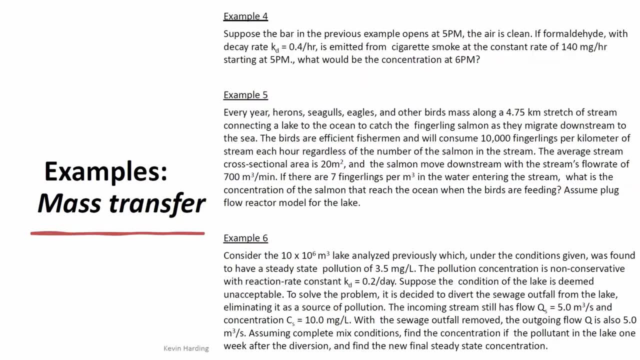 what you might find in a test or an exam. So there are three examples and another three examples to give you another six that you can work on in your own time If you do them you don't. This is just something so that you can get an idea of what to expect. The next one that I need you to know: 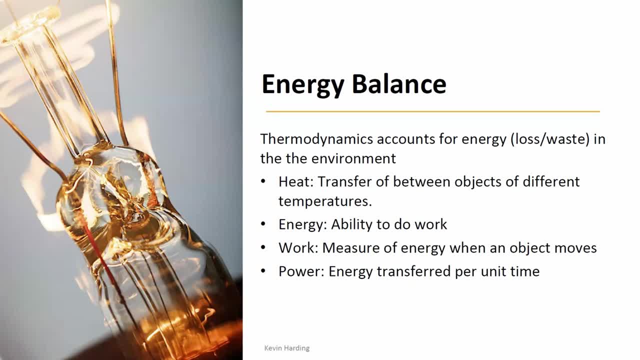 is the energy balance. So the energy balance: I'm not going to ask you detailed energy balance questions. I'm going to ask you very basic questions on the energy balance. So if you probably all your thermodynamics courses or you have some idea of what thermodynamics is, 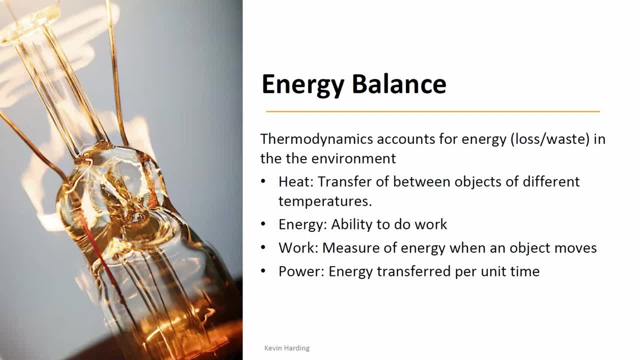 from chemistry. it's not going to be that course where we ask in-depth questions of heat energy, work power. Okay, We'll get to some of that we might ask in a bit. But to start on the energy balance, in the same way that the mass balance has a conservation law, Okay. So the same way that. 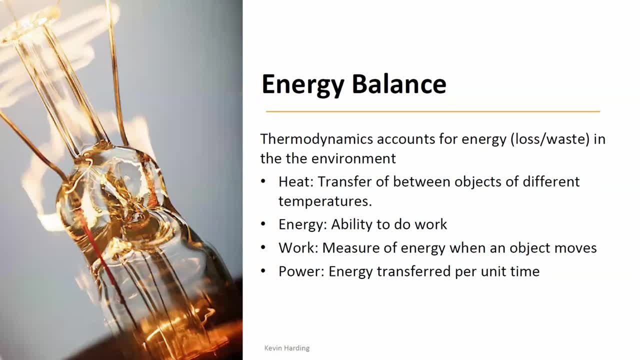 we've got- Okay, Thanks, Big Blue Button. So in the same way that we had for the mass balance. it's a conservation law, So the conservation law will say that anything going in goes out. The same thing happens with energy, So energy is slightly 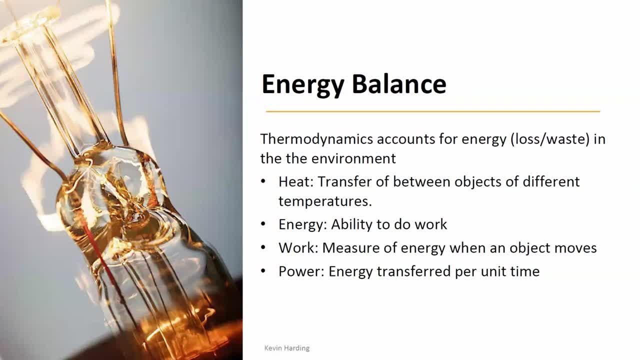 more complicated in that there are different types of energy And there are effectively three that we would ever look at in your thermodynamics courses, The first being heat, which is a transfer of- Sorry, Transfer between Transfer of energy between objects of different temperatures. So if we have 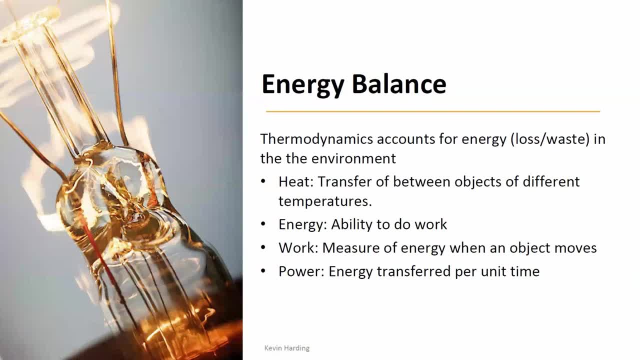 a heat, a temperature gradient. we will have heat from flowing from one to the other. Energy, in its basic form, is the ability to do work, while work is the measure of the energy when an object moves, So work will typically be shaft. 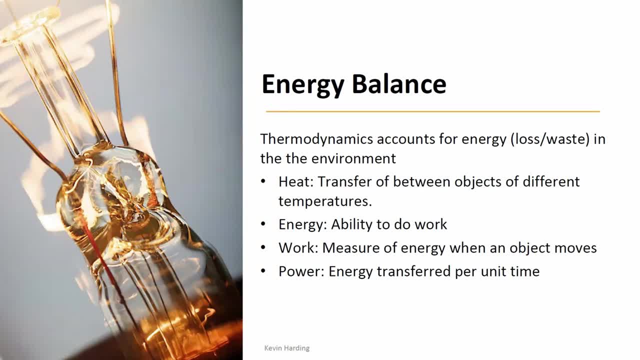 work When something turns around- a pump, a turbine, a compressor, when there's movement involved. that is what work is: Power I've thrown in there, which is simply an energy that is transferred per time, So sometimes you will see energy terms being given per time strictly. 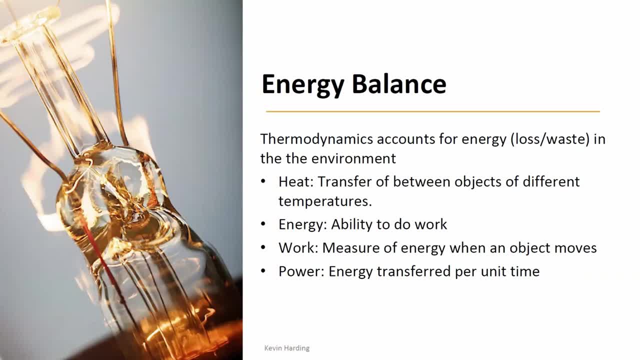 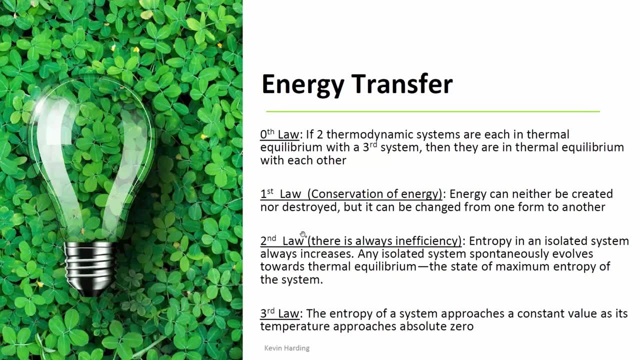 speaking by definitions, that is actually power, because it's by unit time. When we look at energy transfer or energy in general, there are three laws of thermodynamics. So the zeroth law says that if two thermodynamic systems are each in thermal equilibrium, so if there's two objects, 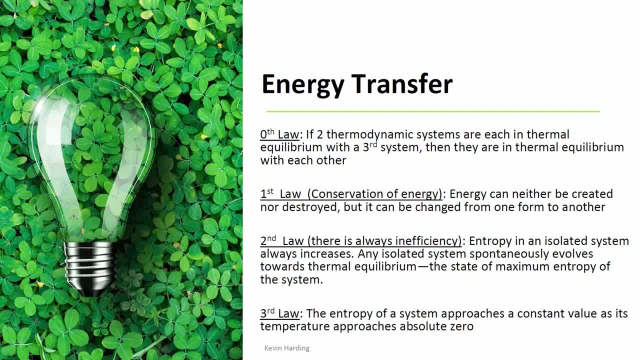 that are at the same temperature. that's what they mean- and they are also in equilibrium with the third. or if there are two, sorry, if there are two thermodynamic systems which are each in thermal equilibrium with the third system, so that means they're the same temperature. 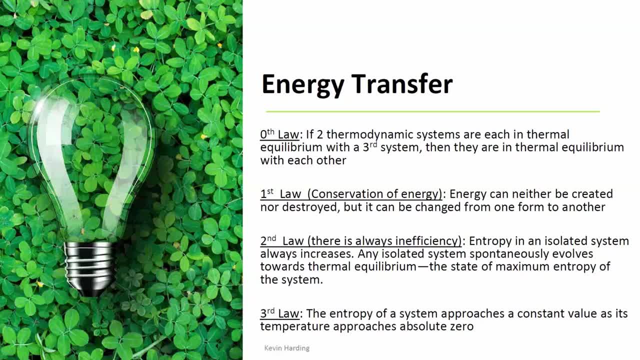 that means they're also in thermal equilibrium with each other. So I think that's a little bit obvious. If I've got two objects that are both at the same temperature as a third, that means object one and two are also at the same temperature. That is the zeroth law, The first law, so the zeroth law. 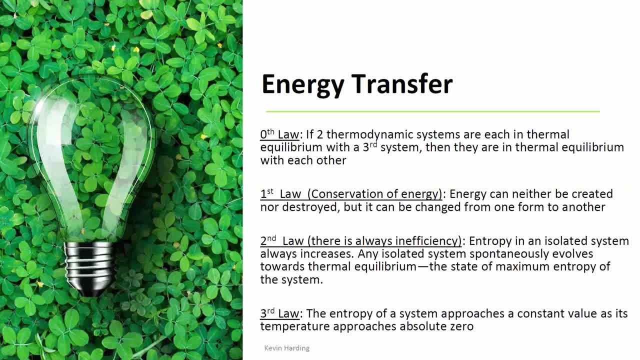 we're never going to worry about now. it's just so that I could complete this list. The first law is the conservation of energy, and this is the only one that we need to worry about for this course. So the conservation of energy is: energy in equals energy out. In other words, means that energy can never be created or destroyed. 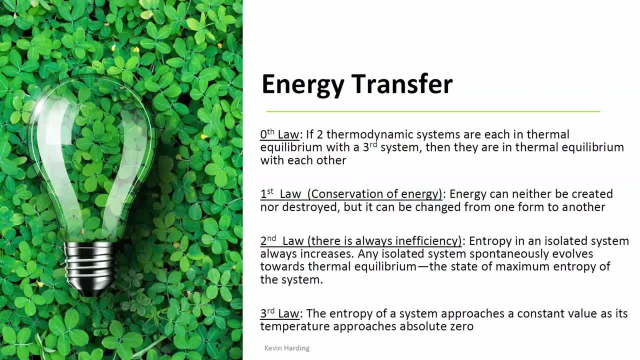 All we do with energy is we transfer it from one form, we change it from one form to another, So we can change energy from heat to work and back again to energy, and that's the one that we talk about with the energy balance. However, law two says there's always going to be inefficiencies. 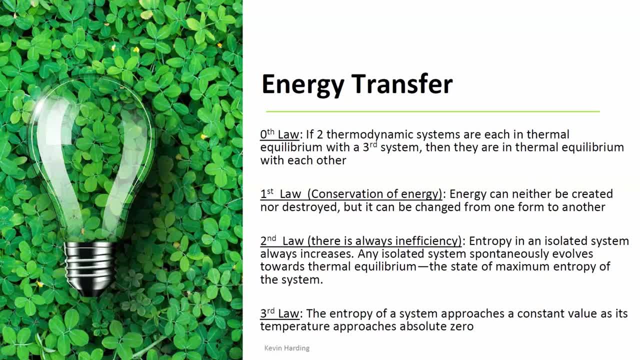 So with that inefficiency we mean that entropy in an isolated system will always increase and any isolated system will spontaneously disappear, simultaneously evolve towards thermal equilibrium. OK, the state of maximum entropy. We will not worry about entropy or the second law or the third. 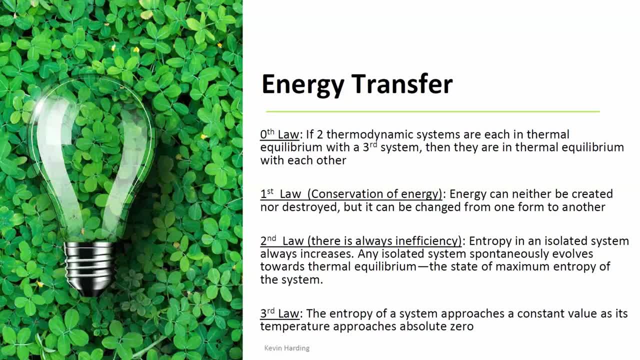 law which states that the entropy of the system approaches a constant value as a temperature. So we're not going to worry about the second or the third law. so this course, you will never see the word end on this page. We're worried about third law, second law, zeroth laws. We're only. 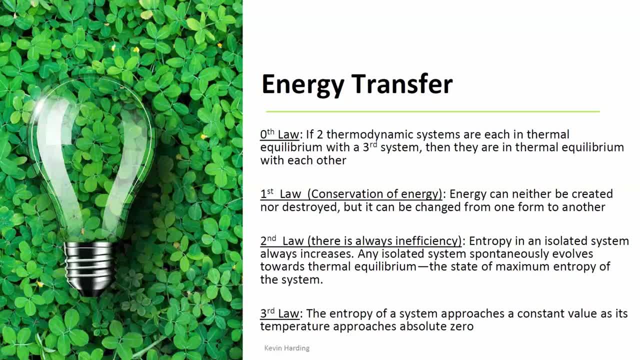 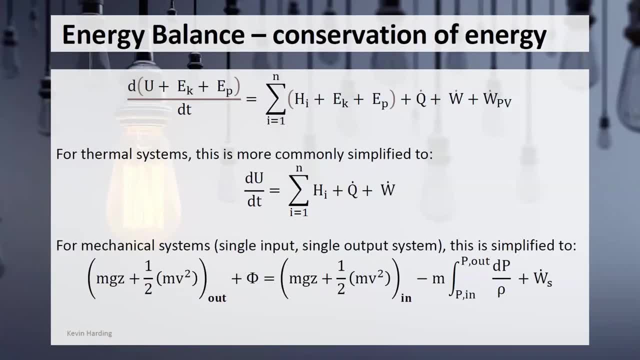 worried about the very basics of the energy balance. OK, as I say, we will get to the details of that in a little bit. OK, just so that I can put up a reminder for those of you that haven't seen it, or a reminder for those of you who have seen it, or just. 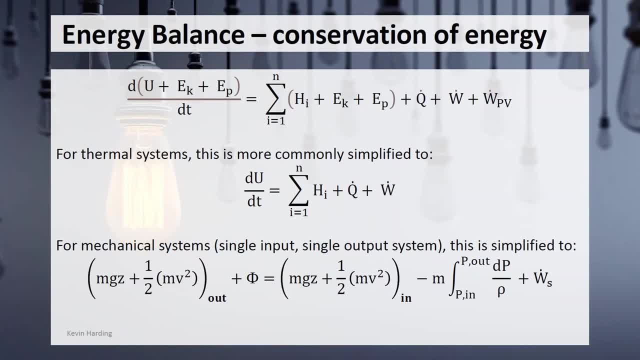 to introduce you to the energy balance, Again, we have a DDT term, So the general energy balance- one at the top is the change in the internal energy, the kinetic energy, the potential energy over time On the left hand side. 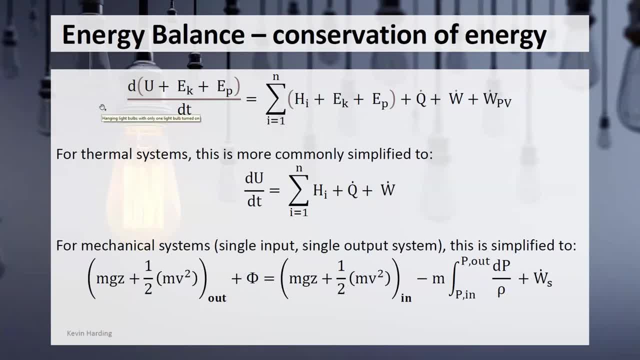 this refers to the system. So if we are looking at a system boundary, whatever is happening inside the system boundary? that is what we're talking about on the left hand side. So the internal energy inside changes. The energy is kinetic. Kinetic energy can only change if the system moves. 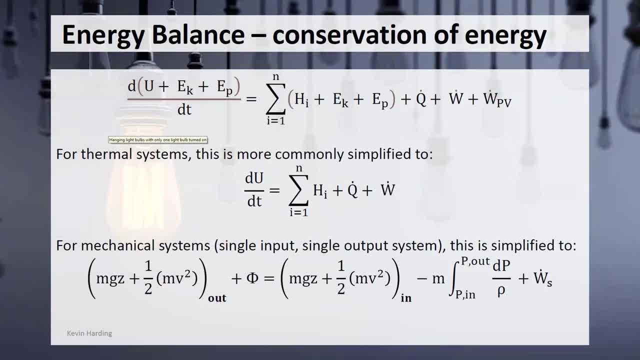 So there's some speed involved and that changes over time, So it's not a constant velocity system. It would be something that is accelerating or decelerating And the potential energy also changes over time, So it also has to be a moving system that. 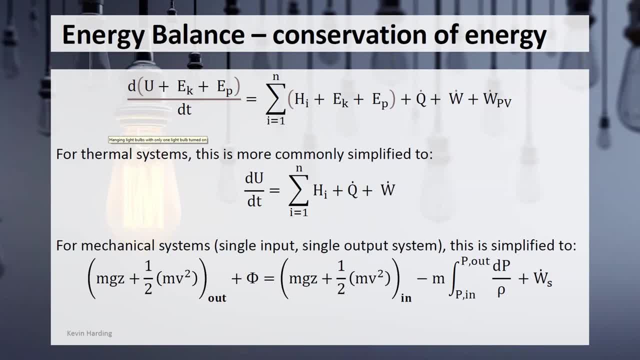 changes. So those all refer to the steady state terms, That is, of the system. On the right hand side we have something similar to what we had with the mass balance, where we now have the summation term. So it's the sum for I is equal to. 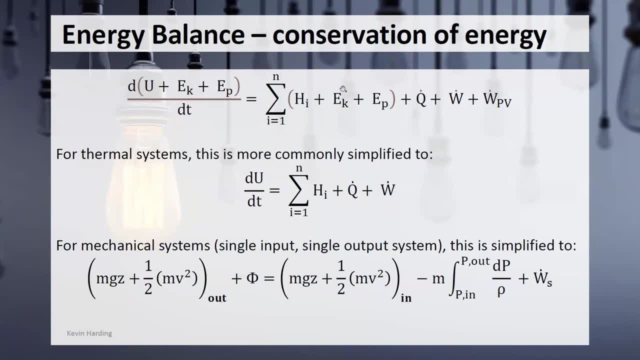 1 to N of these terms here, So H, I, K and E, P. Each one of those are referring to streams into or out of the system, So the enthalpy, that is the energy of the system, of the stream itself. E, K is the kinetic energy, and 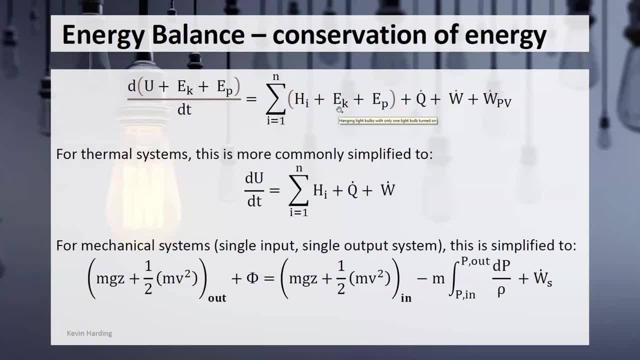 E is the potential energy. So the stream coming in on the left hand side, the gas coming into that system, might be at a different velocity to the stream that's going out. The same thing with the potential energy. it may have a different height. So you might have something. 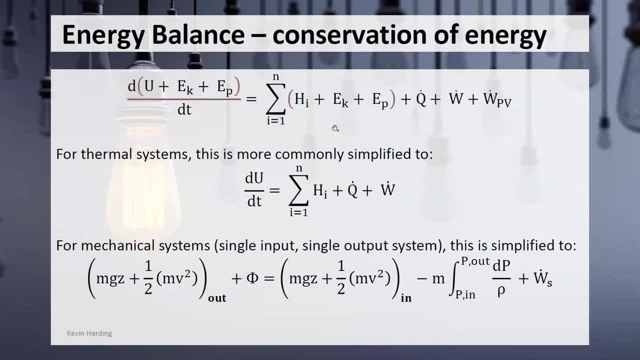 going in at a low position and coming out at a high position. So this will be a change And those are the streams coming in and out. There will be any additional heat in the system if you're under it, If there's a furnace and you're heating something in the box. 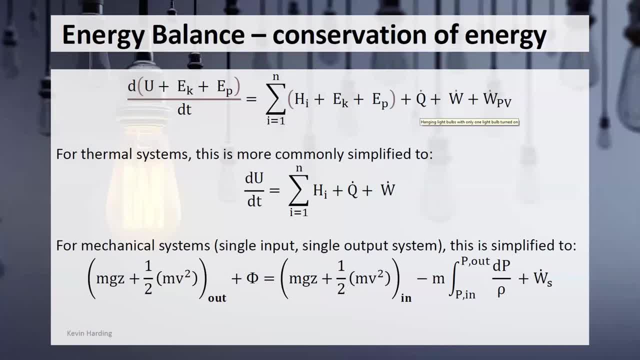 that is the Q term. Heat is going in or I see there are various people typing messages to me. I hope there isn't a problem. That is the heat And the work term. there's W and WPV. I would typically write this, probably as: 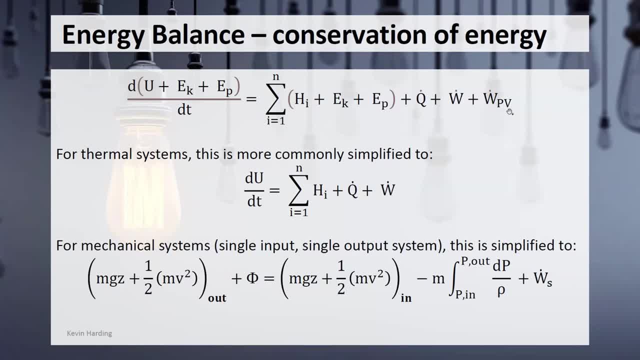 one work term. So the W term is all works. E textbooks would write E, so that's the work. due to a change in pressure As a second term, I would typically write that as one term For simplification. this comes down to: 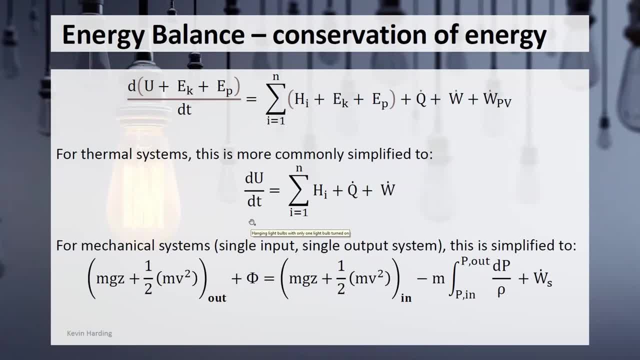 if we're looking at thermal energy, we're looking at thermal systems And we said that in this course. almost all of you can't hear me clearly. I'm not quite sure what to do with that. That might just be a connection issue. 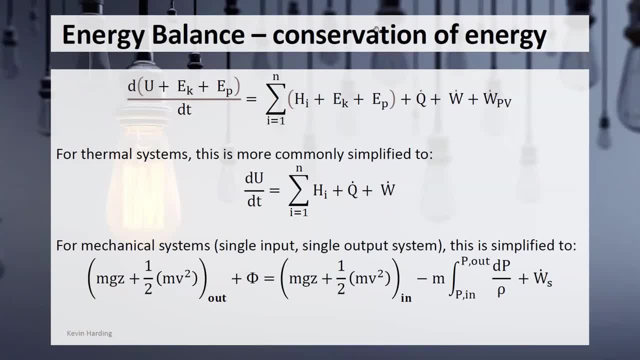 which I'm trying to see if I'm connected. Unfortunately I'm not, as much I can. We said, of course, most of the systems are going to be thermal systems, So thermal system, this would more simply drop down to change in internal energy. 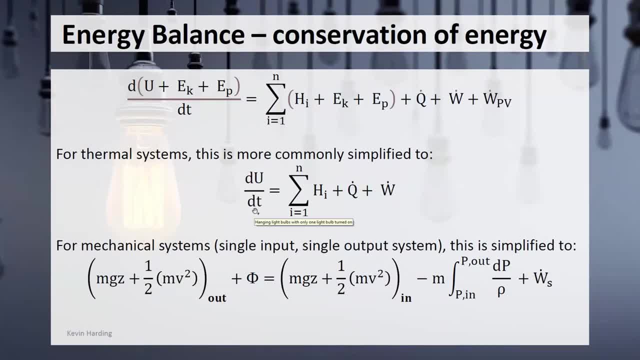 and change in time. So there are not many systems in terms of the heat and there are not many systems in terms of the temperature in general. So the heat is a value that's P, so I think It's the heat of the system. Let's put heat into terms. So that's where P comes in And that's where the heat comes in. So you're on the next slide. So the other thing is: is we're looking at extremely high energywhat other elements do? 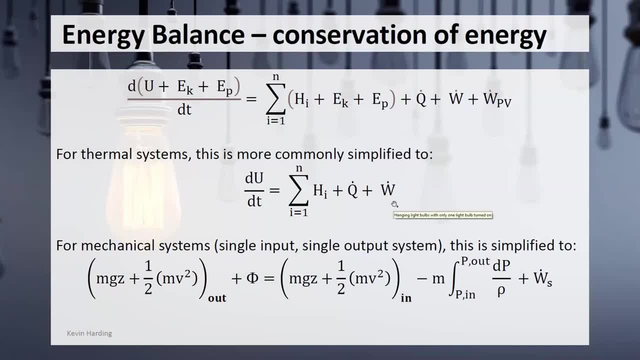 Okay, This is my reminder, for those of you that have seen it before, that we can also have mechanical systems. With mechanical systems, we can rewrite the DUEKEP term, where we only look at the EK and the EEP, If we have a steady state system with only a single out, the thermal terms. 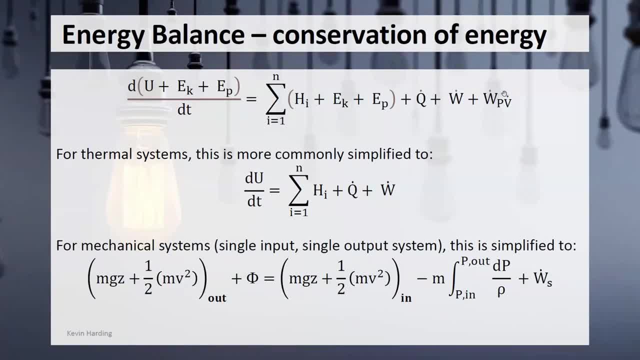 of HIQ fall away. The WPV will remain in place. Sorry, no, the WS, sorry, the WPV will fall away. The W, the work term will only be shaft work, which becomes WS at the end of this term. 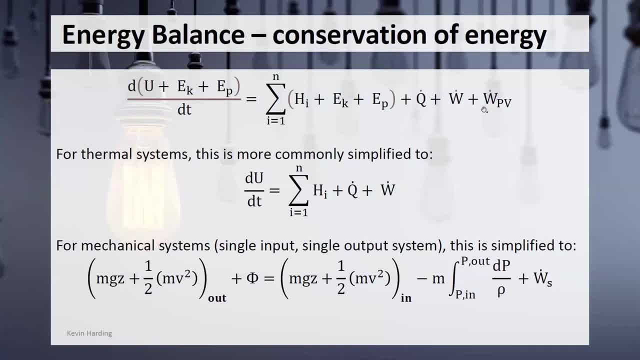 You write that as that equation at the bottom In this course. you do not need to know anything about this bottom equation, Okay, So just to clear that up. you do not need to know anything about the bottom equation. I'm also never going to ask you about the general energy balance equation. So what I've 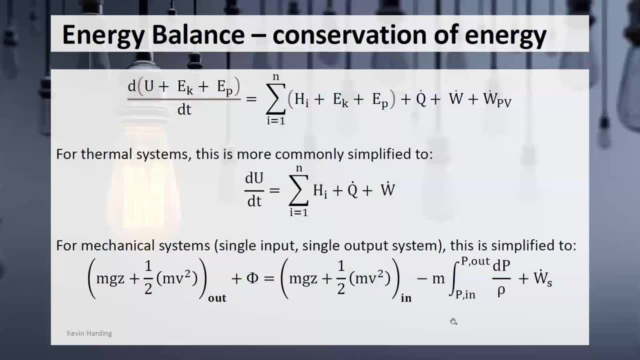 pretty much done for you now. you're not going to be examined on The only thing that I might examine you on. so I'm just trying to see I've got something wrong on my screen here. The only thing I might examine you on is going to be in terms of the heat of vaporization. So 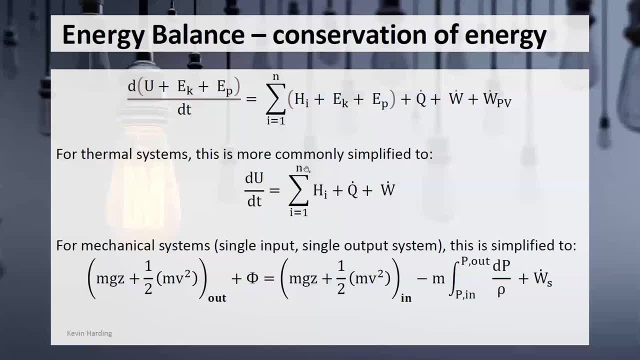 you'll see. there's one question on heat of vaporization which I'm sure you've all come across in your 20, 21 course or in first year already. So if there's a certain heat added to water, what is the evaporation that comes onto that? So you're going to see some questions in the 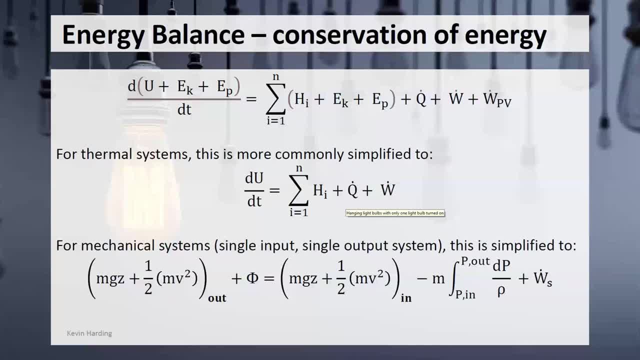 TAT, as well as some of the other examples that are going to make you think of this energy balance. In actual fact, there are mass balance questions. They are not energy balance in terms of this slide. So, to simplify it for all of us, you're never going to have to worry about this slide. 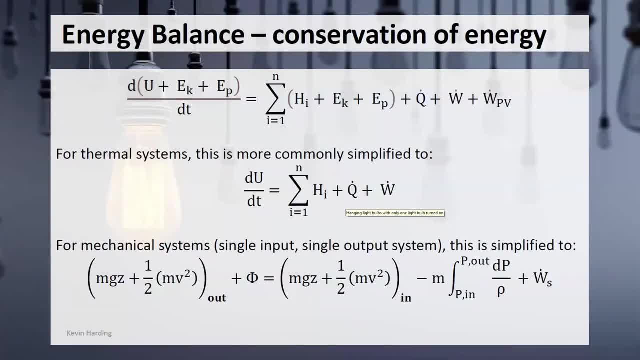 again. Okay. I do need to highlight this, though, because questions in the text book are going to start referring back to these equations, So if you want to know where these equations come from, it's from the start. Sorry, They're going to come from these equations that. 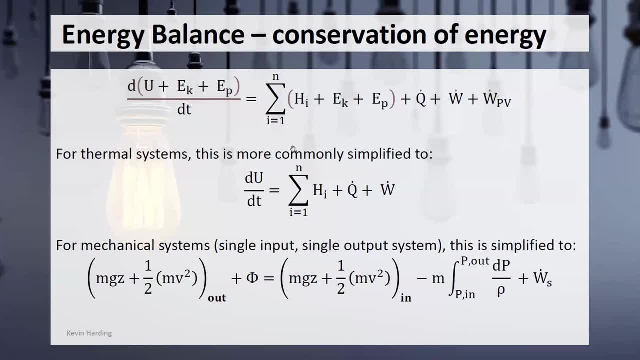 simplified, So some of them start out quite complicated, but for your sake, you only need to worry about the mass balance. Okay, And I'm stuck. Sorry, I can't change slides. Okay, They are all. also going to be some examples where there is going to be heat transfer. 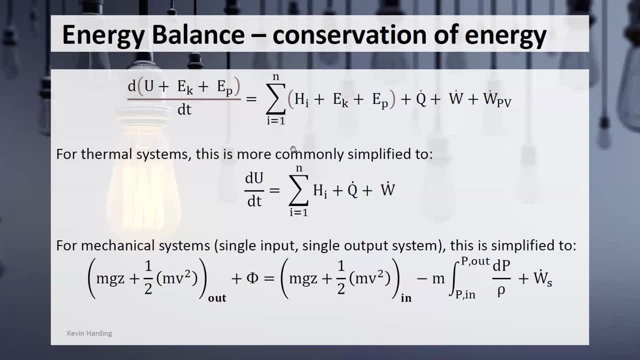 Heat transfer was not a prerequisite for this course as well. So in that textbook if you come across questions on heat transfer, you do not need to worry about heat transfer. So the only thing that you need to know about the heat transfer is that they are heat transfer. The first one is: 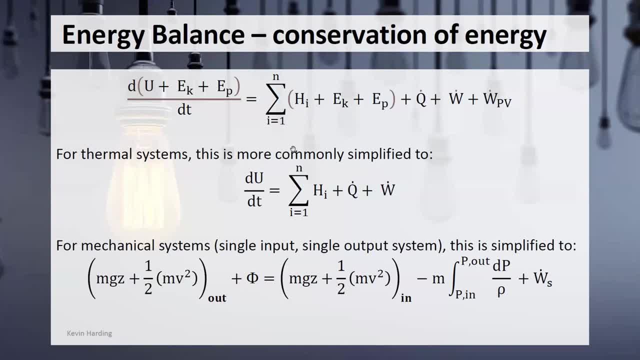 conduction. So there's the equation for conduction, which probably all have seen somewhere before. There is convection to change in temperature, So you don't need to worry about the heat transfer on convection either. And the last one is if there is radiation. So there are a lot of questions on 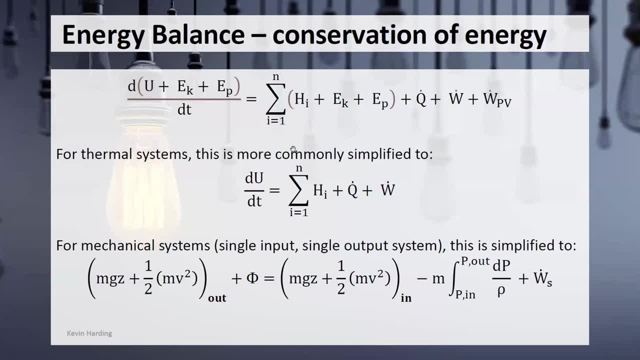 radiation in the textbook. I don't need you to worry about the heat transfer when it comes to radiation either. Why I'm putting this up here and reminding you all about it is because, depending on what your other lecturers do in their courses, so they are. 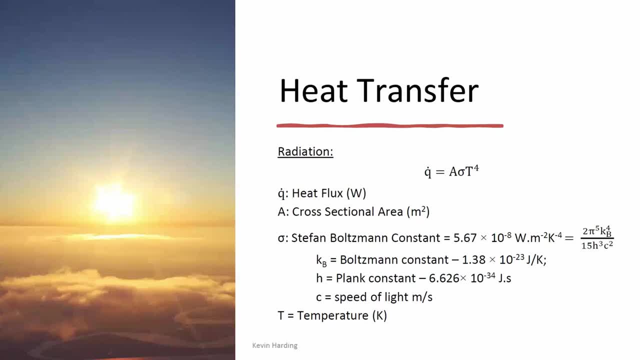 definitely know they are energy or their thermodynamics courses. for every student involved in this course There's also going to be some heat transfer type material definitely for, I think, all of you as well. The questions that they ask in that section could be more. 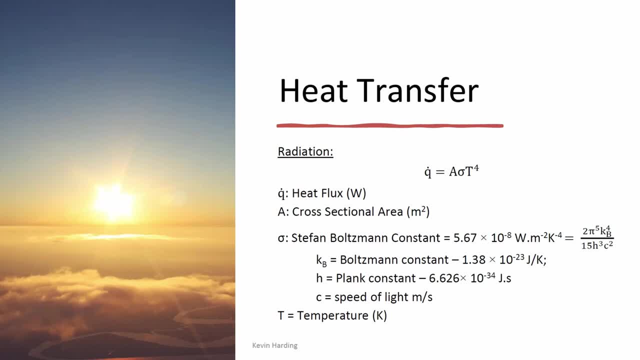 on a environmental engineering type slant, just because of the example they use. Okay, So you could get questions in your other courses on a word, a word sum, basically a word problem that is going to be used in your other courses. So if you have any questions, please feel free to. 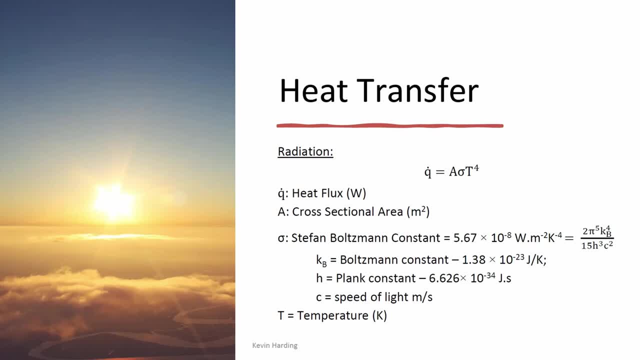 put them in the Q&A box and we'll try to answer them. So I'm not going to be asking you to solve heat transfer and energy balance questions in this course, but in your other courses. they might use environmental engineering examples in those courses, Please remember. 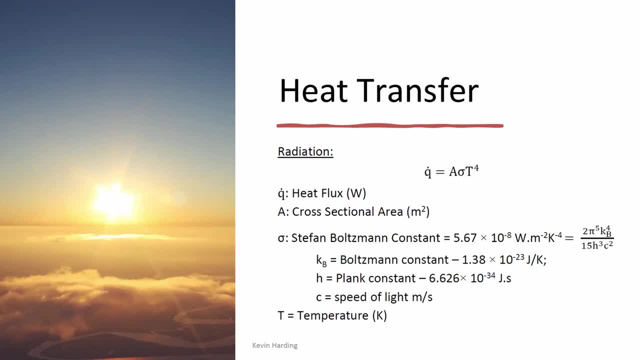 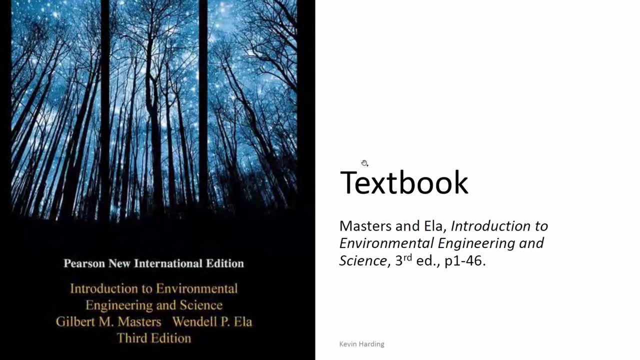 that the two courses do talk to each other from that sort of side of things. Okay, As I said at the beginning, this section now starts with the textbook. So those of you that have the textbook- and I'm hoping all of you have access to it at least-